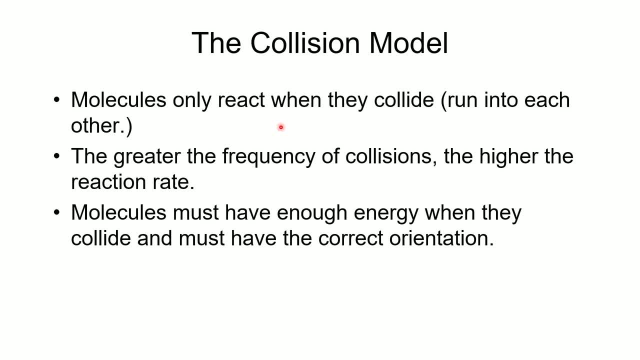 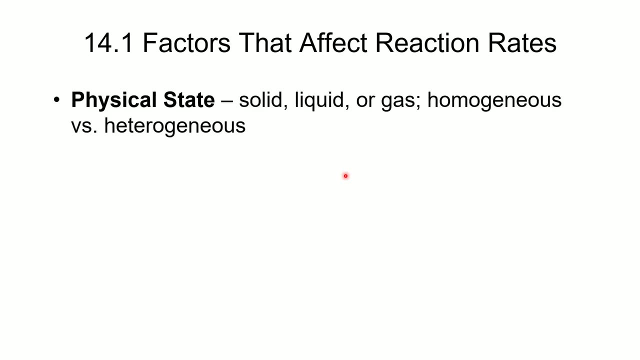 run into each other and they need to have the correct orientation. If they don't have the correct orientation, then they might not react. So we want to look at four main factors that will affect the rate of a reaction. One is going to be the physical state. We'll talk about solids. 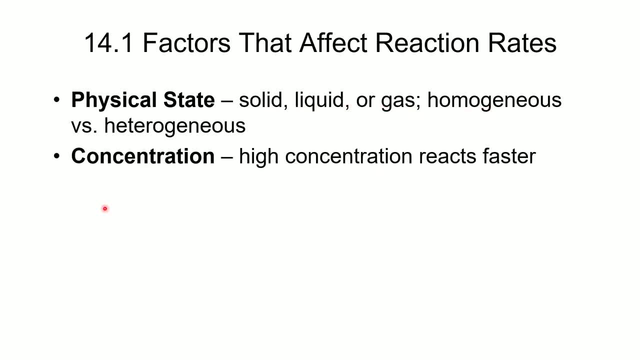 liquids and gases, and homogeneous versus heterogeneous. The second is concentration. The higher the concentration, the faster the reaction. The third thing is going to be the temperature. Almost always, if we increase the temperature, the reaction rate will increase as well. And then, finally, the presence of a catalyst. By adding a catalyst, 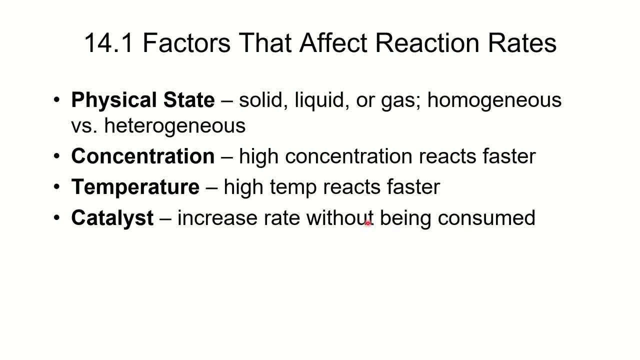 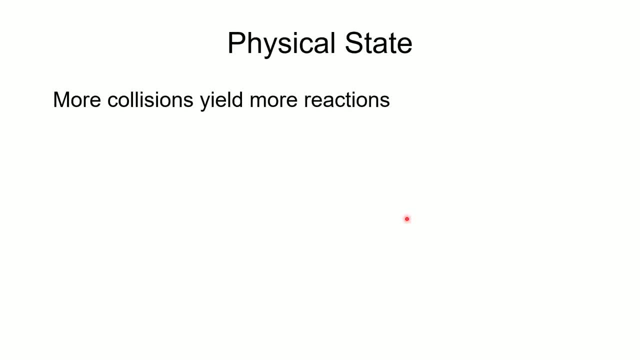 we change the mechanism of a reaction and the catalyst ends up not being consumed over the course of the reaction. So let's start with the physical state. Again, the collision model tells us that more collisions should give us more reactions. Well, we'll find that gas phase. 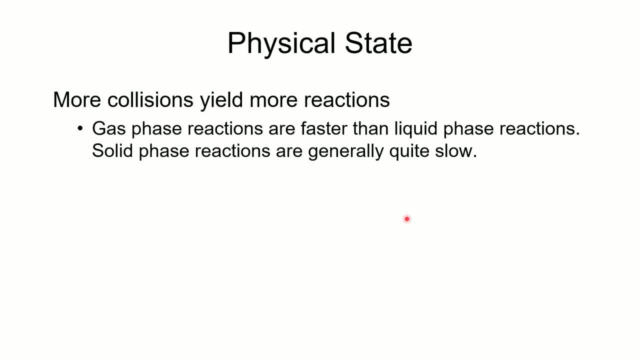 molecules are going to be moving more freely and running into each other more often than the liquid phase, so gas phase reactions will go faster than liquid phase reactions. Solid phase reactions go very slowly because the molecules aren't really moving around very much, so they 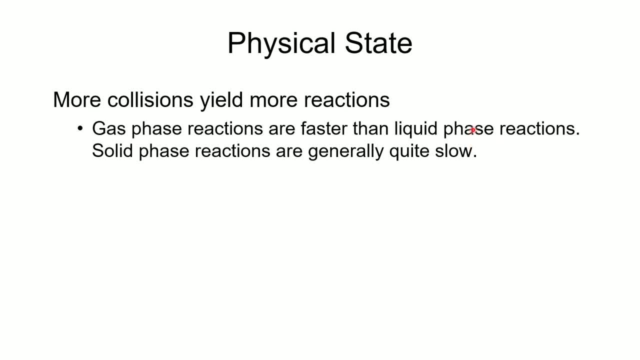 have trouble running into other molecules. Now, certainly they run into the adjacent molecules, but in order for it to react with something else we would need to move those molecules around. So we'll find that almost always gas phase reactions go faster than liquid. 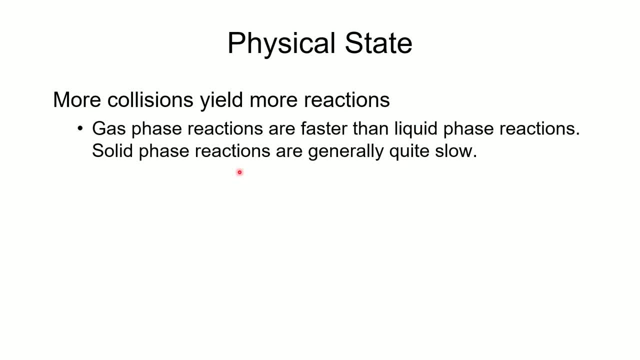 and liquid goes more, Much, much faster than solid. When it comes to homogeneous versus heterogeneous reactions, well, in a homogeneous reaction, the molecules are all in the same phase, so they're more likely to run into each other and they're more likely to proceed quickly. In a heterogeneous reaction, however, 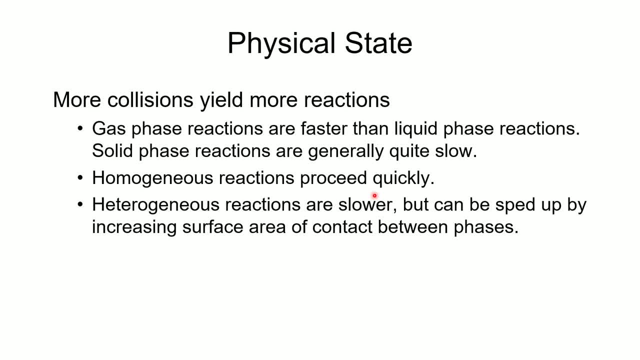 we'll find that they go much slower because the molecules don't run into each other as often. Now we can speed up the rate of a heterogeneous reaction by increasing the number of collisions that we have. We're increasing the contact area between the phases, but there is a limit to that. 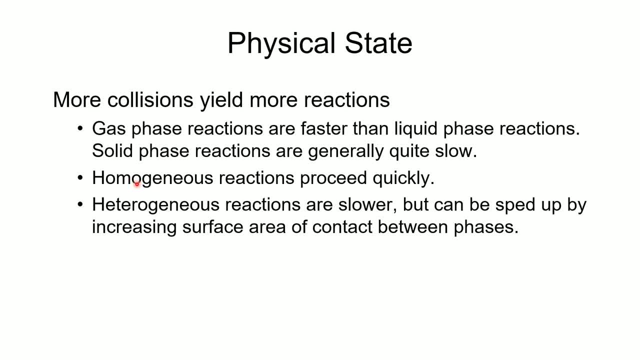 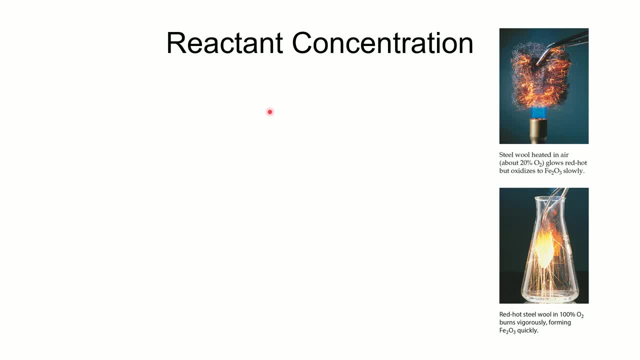 So we'll find that if we really want a fast reaction, we're going to do a homogeneous reaction. Our next factor is reactant concentration. Again, generally speaking, increasing the concentration increases the number of collisions and by increasing the number of collisions, 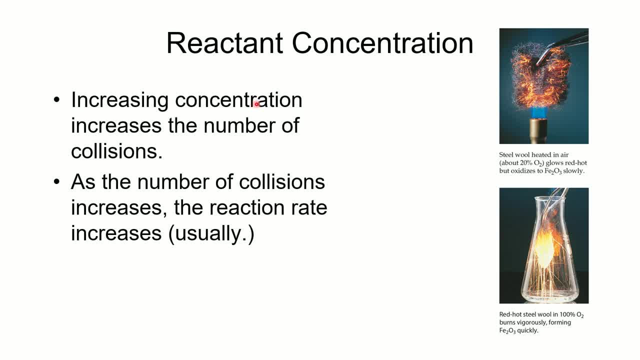 we'll increase the rate of reactions. So an example of this is the steel wool that I have over here on this top picture. It is in air and since air has a concentration of oxygen at about 20, 21 percent, at about 21 percent we'll find that the reaction goes fairly slowly. 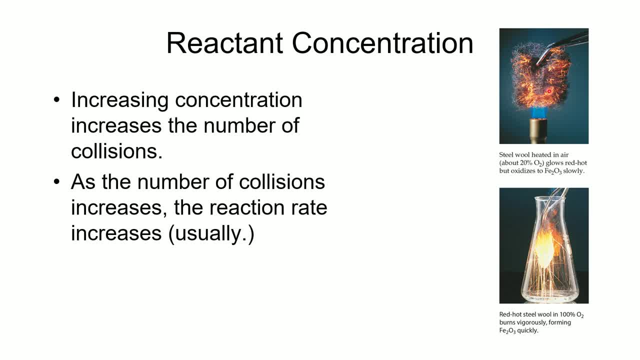 So the iron that is in the steel wool will get oxidized, but it goes fairly slowly. If, however, we take that burning piece of steel wool and plunge it into pure oxygen, the reaction rate will go much, much faster and burn much more vigorously. 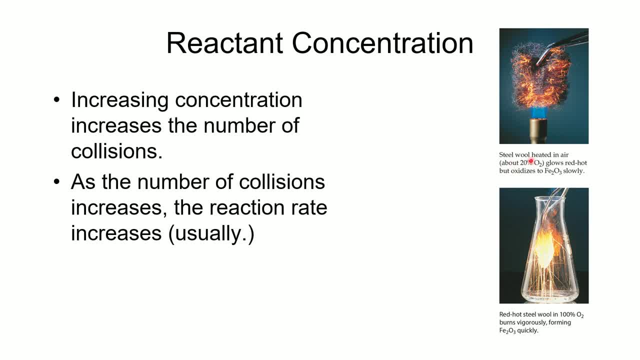 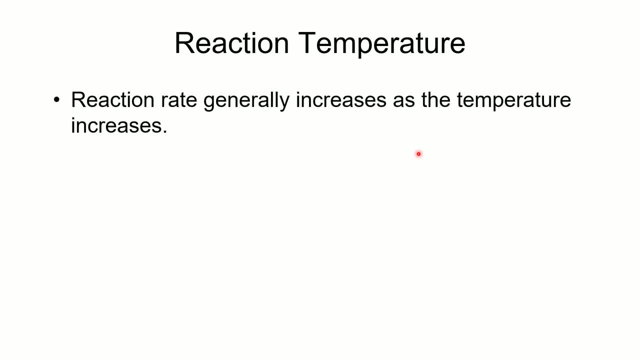 So that's always a fun experiment. Alright. so now for reaction temperature. Generally speaking, if we increase the temperature, we will increase the rate of the reaction. The reason behind this is that at higher temperatures the molecules move faster and therefore they run into each other more often. 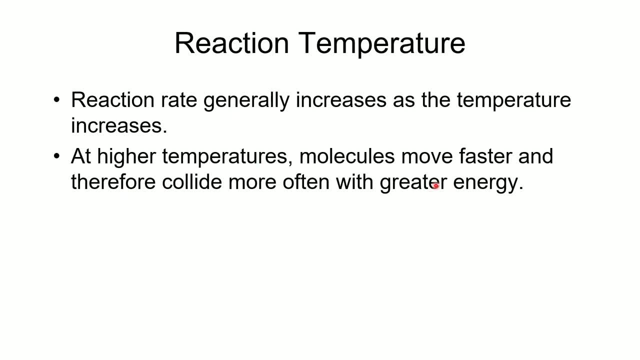 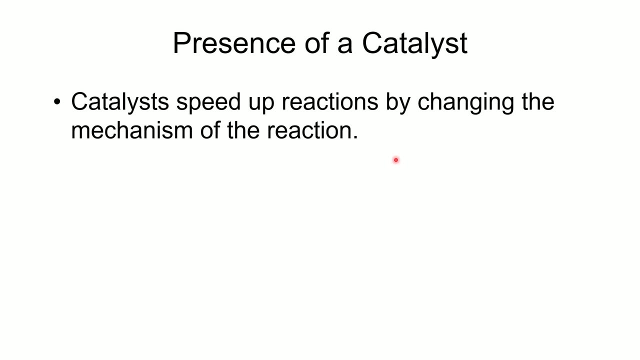 And when they run into each other more often, they also have greater energy. So increasing the temperature is a sure-fire way to increase the rate of reaction. And then, finally, our fourth factor is the presence of a catalyst. Catalysts will speed up the rate of the reaction by changing the mechanism. 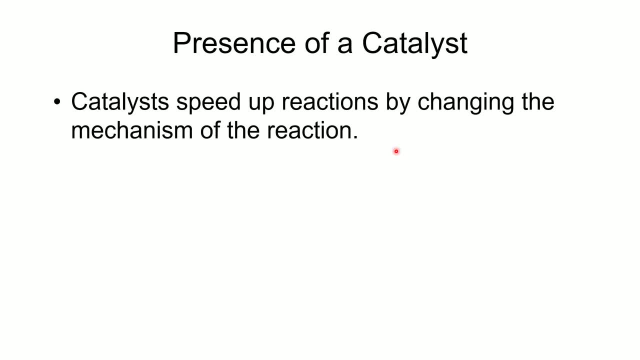 Now, catalysts are kind of special And they do some really cool stuff. So we're going to look at that in more detail at the end of the chapter. But one of the key features of a catalyst is that a catalyst is not consumed over the course of a reaction. 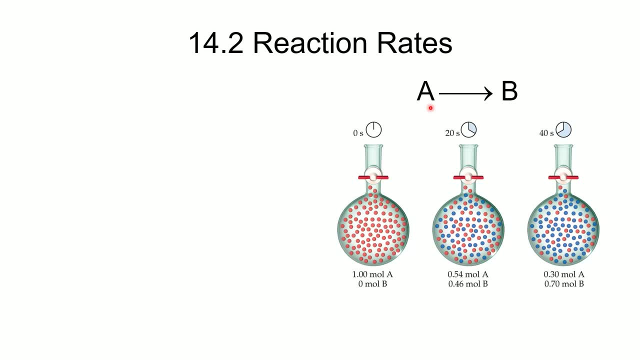 Alright, well before I can show you how these things affect the rate of reaction particularly, we're going to spend a lot of time today, particularly we're going to spend a lot of time today, talking about how concentration affects the rate of reaction. 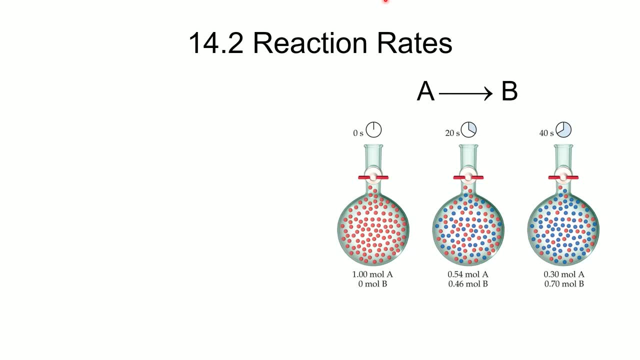 But before we can really dig into that, we have to know how to measure the rate of reaction, And that's going to be our primary goal here today. So the rate of reaction can be determined by monitoring the change in concentration. the change in concentration. 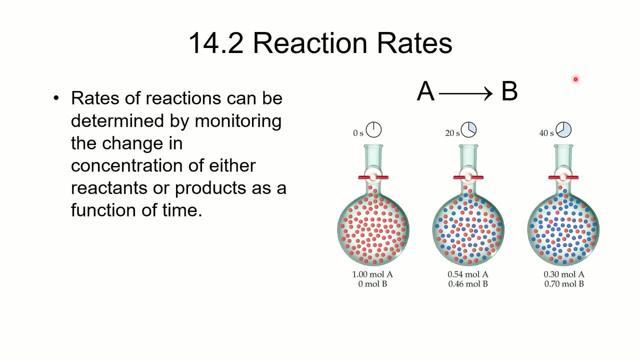 of the reactants or the products, if we want to, as a function of time. So here we've got the reaction where A is getting converted into B. You'll notice that at 0 seconds we've got 1.00 molecules, or moles of A. 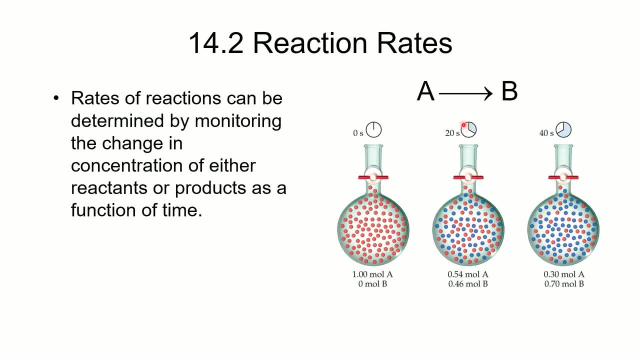 and no moles of B. After 20 seconds we've got 0.54 moles of A and 0.46 moles of B, And after 40 seconds it's down to 0.30.. And after 40 seconds it's down to 0.30 moles of A and 0.70 moles of B. 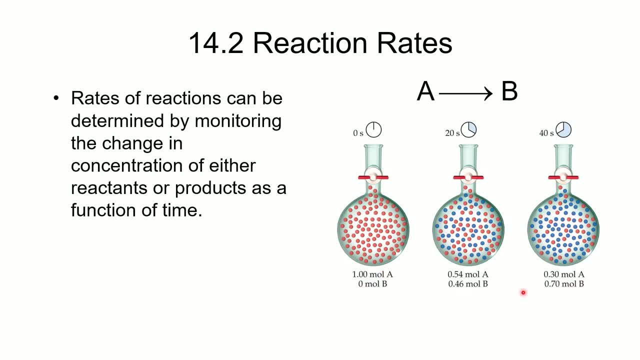 So you'll see that the A is decreasing and that the B is increasing. Now I want you to give me an estimate of how many moles of A do you think there will be at 60 seconds. So I want you to pause the video and make your best estimate of what you think the number of moles of A is going to be at 60 seconds. 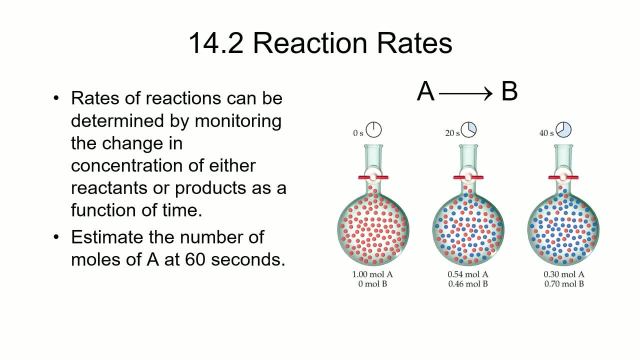 Alright. so now that you've had a chance to give yourself an estimate of the number of moles of A at 60 seconds, let me show you what I came up with. So, between 0 seconds and 20 seconds, we will find that the number of moles of A went down by 46%. 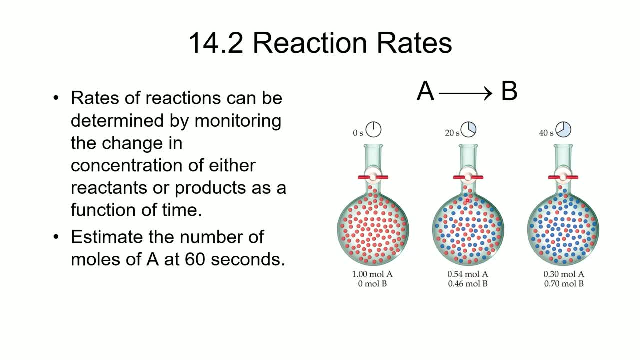 And if we do the calculation, what percentage it goes down? between 20 and 40 seconds we'll see that it goes down by about 44%. We can do that if we take the amount of change divided by the original amount. So we'll do 0.24 divided by 0.54. 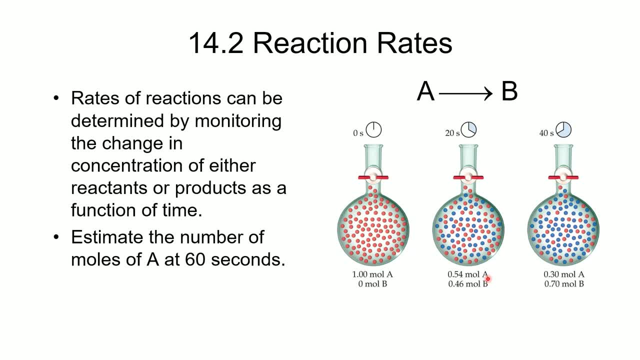 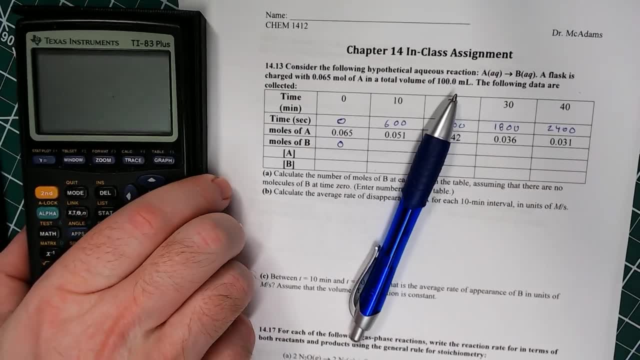 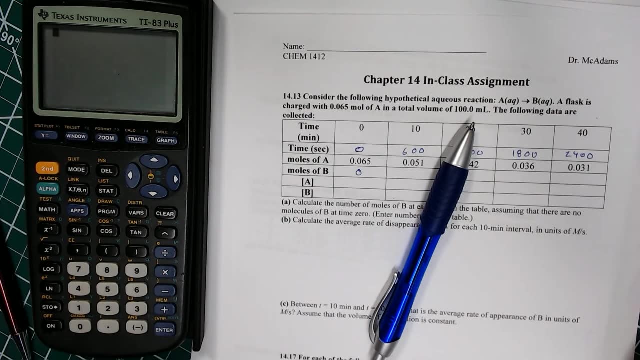 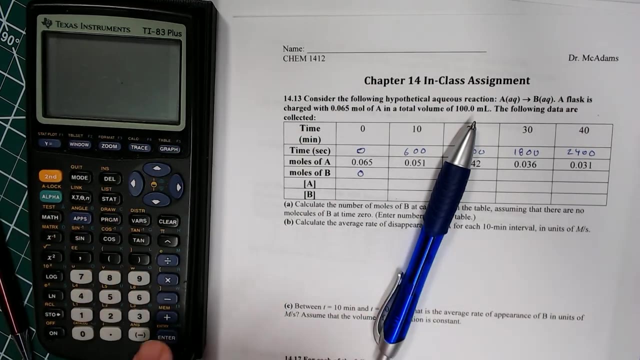 And I'm going to switch over to my camera here. that's got my calculator Alright. so there, I've got my calculator. I'll turn that on, Alright. so now that I've got my calculator turned on, we'll do that calculation. 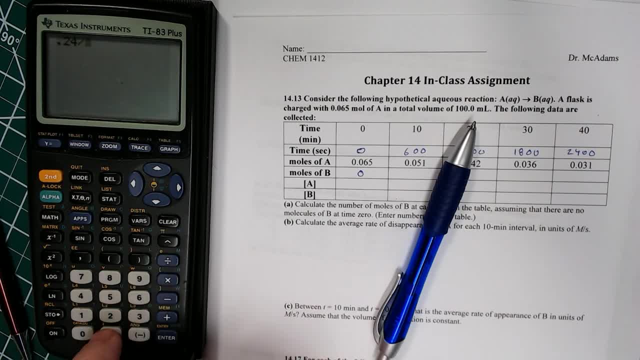 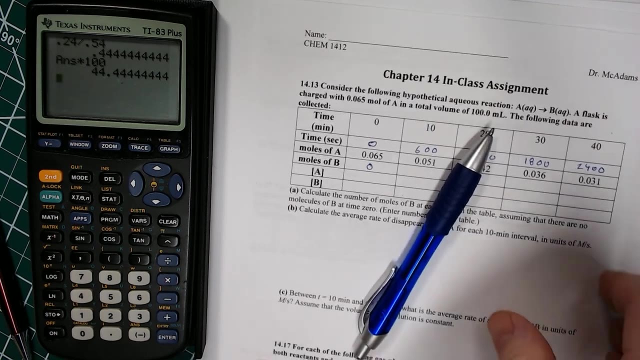 We'll take 0.24 and divide that by 0.54.. Then we'll multiply that by 100 to make it a percentage. You'll see the number. there is about 44%. The first number was 46%. We're going to say it averages to about 45%. 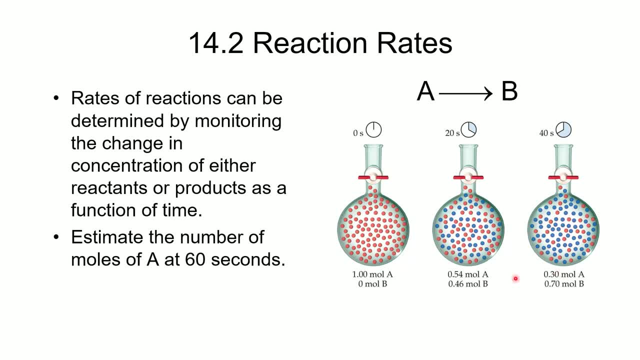 So let's go back to this picture. So here it went down by 46.. There it went down by 44. So let's say that on average it goes down by about 45%. Well, we're going to subtract 45% from that number, from the 0.30. 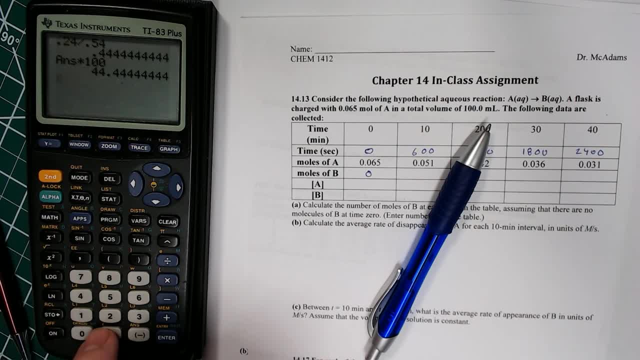 So we'll go back to the calculator And since we're subtracting 45%, let's just multiply it by 55% And that will give us the value. So 30 times 0.55.. And that gives us 16.5.. 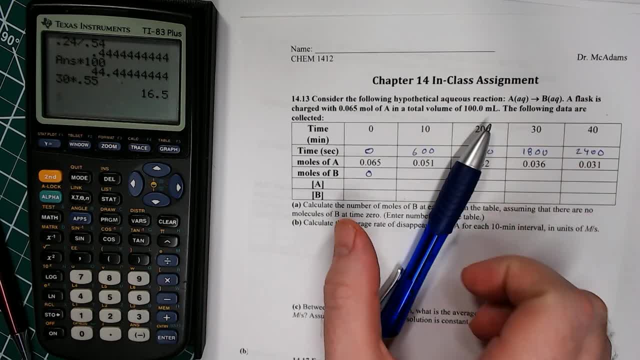 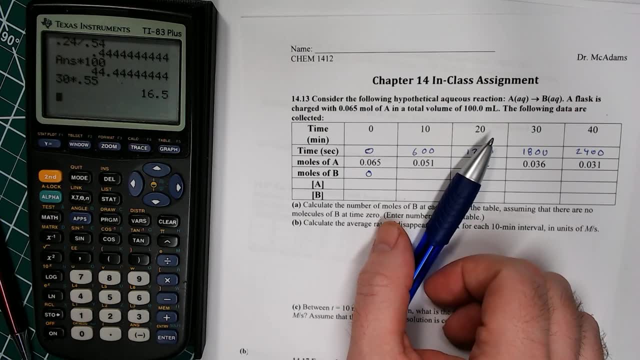 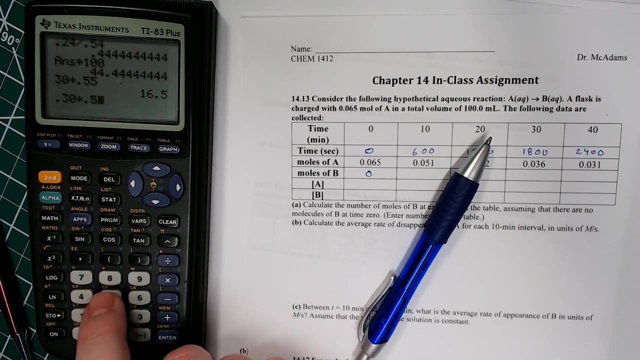 So if you had guessed either 0.16 or 0.17 moles of A, I should have made that 0.30 times 0.55.. So if you had gotten 0.16 or 0.17 moles of A, 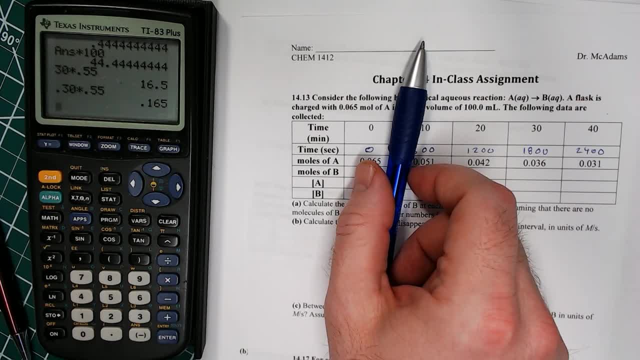 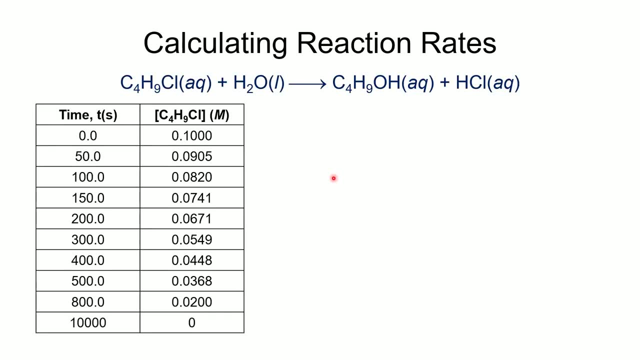 good job, All right. So now we want to look at a real chemical reaction. Instead of having A getting converted into B, we want to look at a real chemical reaction, And in this real chemical reaction we've got butyl chloride that is getting converted in. 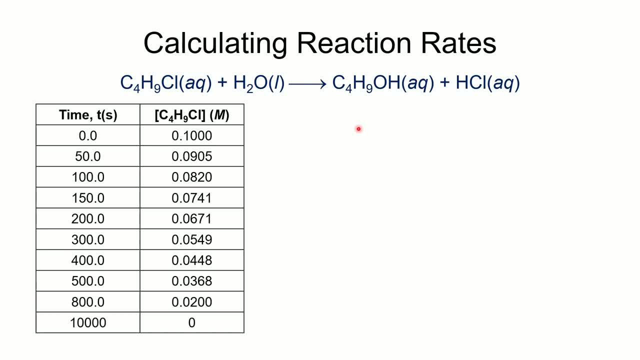 that is reacting with water and getting converted into butyl alcohol plus HCl. So in this reaction, whoever did the experiment, has measured butyl chloride as a function of time, So they picked out several different times and measured the butyl chloride at those times. 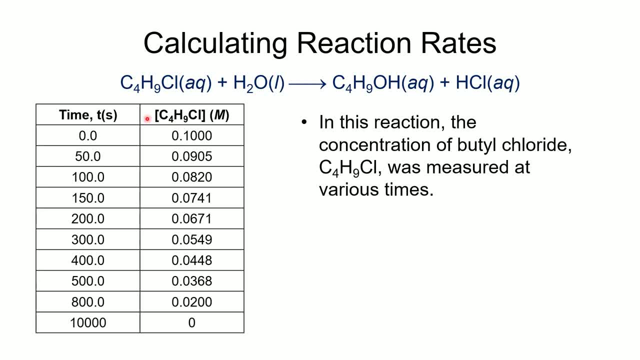 Now on this table. I want to point out something You'll notice here, that we've got square brackets around the C4H9Cl, the butyl chloride. Well, those square brackets, by convention, mean concentration in molarity. 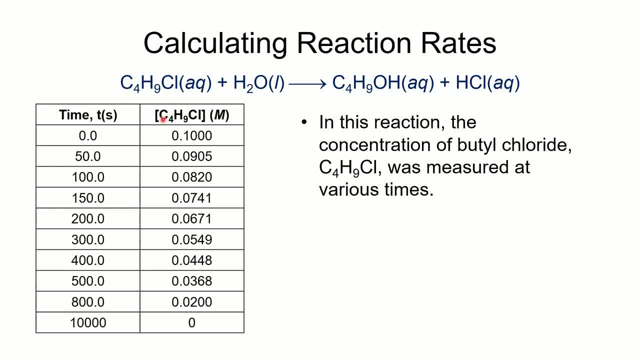 So they mean concentration in molarity. So we're going to use that convention throughout the rest of this course. So I wanted to point it out and make a big deal about it. When it comes to calculating the rate of a reaction, 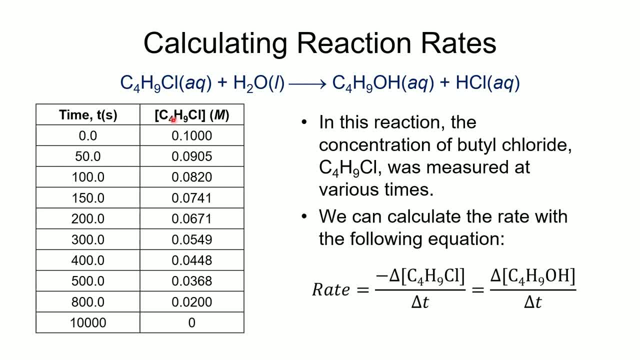 we can use the following equation: So the rate of reaction is going to be delta and of course you guys remember that delta means change, So the change in concentration of butyl chloride over the change in time. Now you'll notice that I put a negative in front of this. 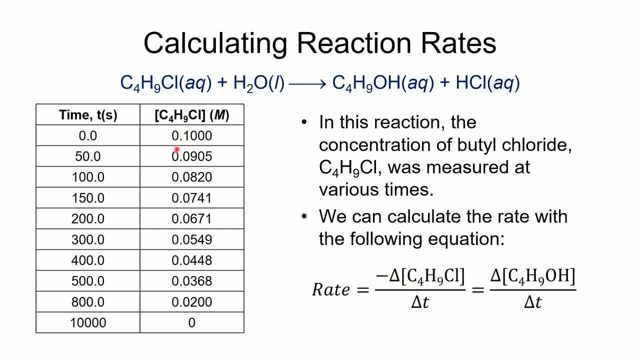 And the reason for that is if we just do change in concentration over change in time, because the concentration is decreasing, we would get a negative value. Well, we want positive values for the rate of reactions, So we simply put a negative out front. 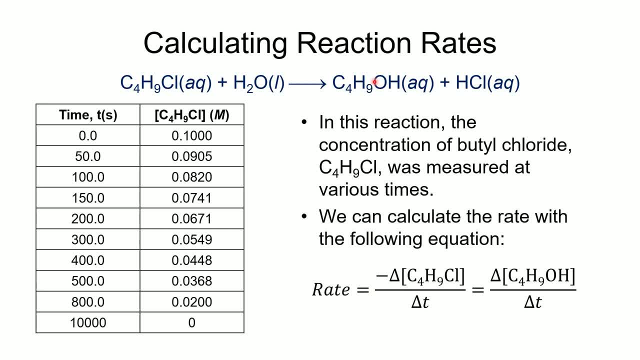 to make that a positive value When we're talking about products. products, on the other hand, are going to increase in concentration, so we don't need a negative value in front of those. So let's do the calculation for the change in concentration of butyl chloride. 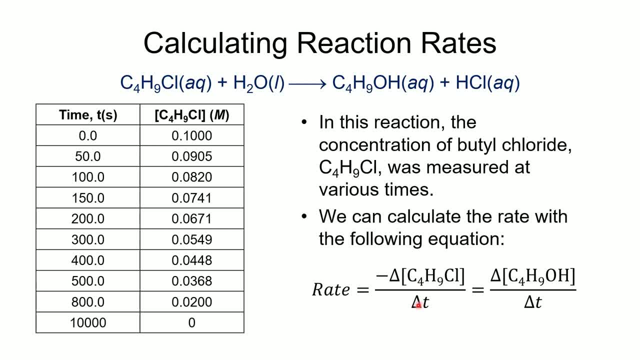 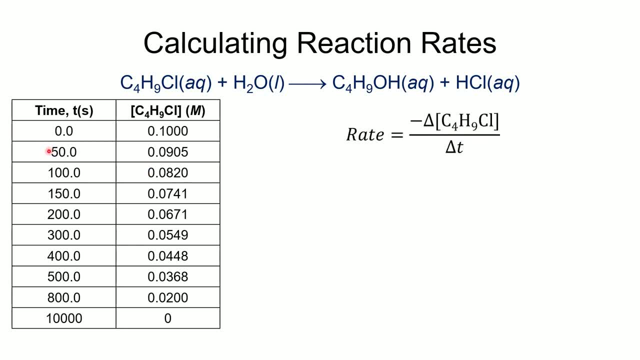 over the change in time. So I've got the data here, Here's our formula, And we're just going to pick between 0 and 50 seconds to start with. So between 0 and 50 seconds. So here is the concentration at 50 seconds. 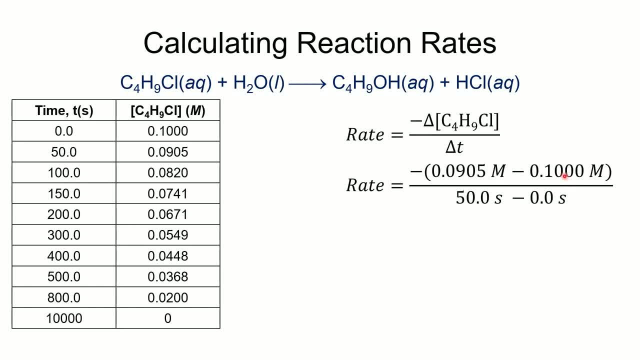 which I put right there. Here's the negative we have out front. We have: .1000 is right there, And then we'll do 50 seconds minus 100 seconds down in the denominator. Well, if you punch that in your calculator, 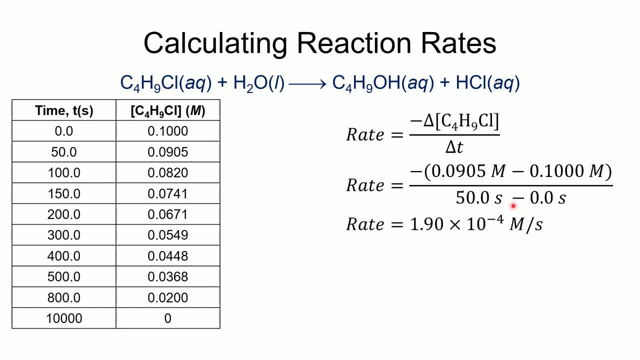 which I encourage you to do- you will get this value 1.90 times 10 to the negative 4 molar per second. Now, throughout this chapter and any time we're talking about reaction rates, these will be our units for reaction rates. 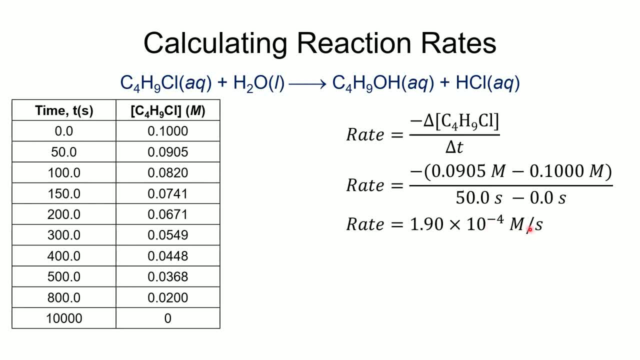 Will be molar per second. So molar per second. So you'll see that we've done that, we've done that calculation And we could do all of these. We could do the calculation between 50 and 100,. 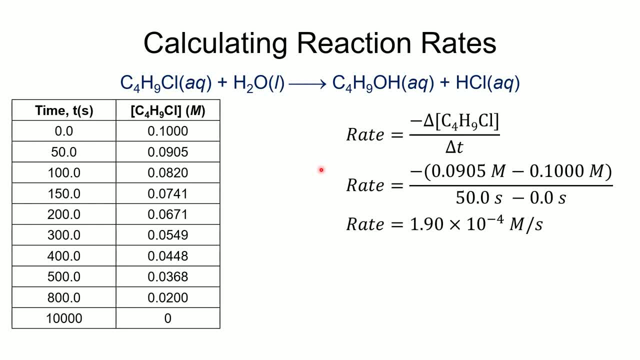 100 and 150. And I've gone ahead and done those and put those values here. So here's that one that we just did. But we can also do between 50 and 100.. And we'll see that it's 1.7 times 10 to the negative 4.. 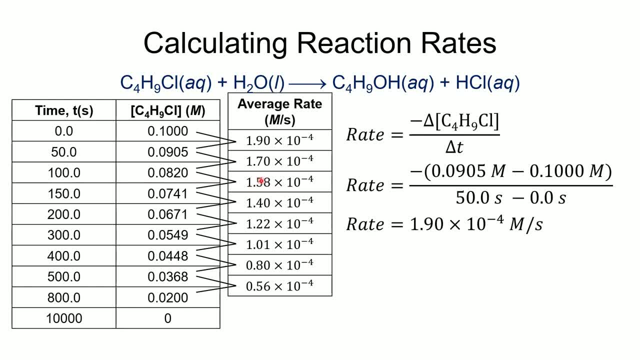 Between 100 and 150, we get 1.58.. So on and so forth. Well, we're going to do this same thing. I do want to point out that the rate of reaction does decrease as time goes on, And we're going to see that that happens. 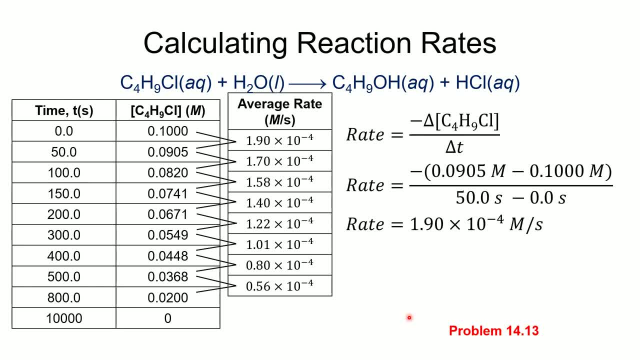 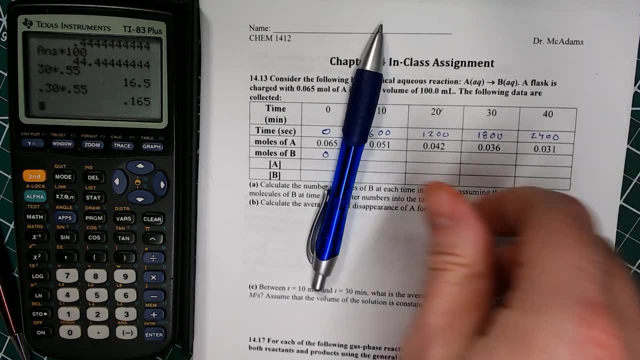 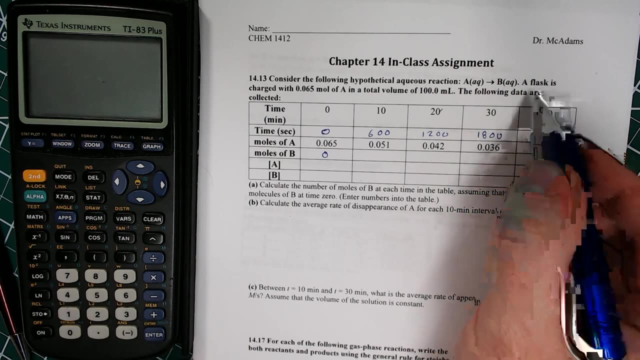 in just about every single reaction that we look at. So we're going to go over to the in-class assignment and do number 13.. Alright, So we have a reaction here where A is getting converted into B. We start with a flask that has 0.065 moles of A. 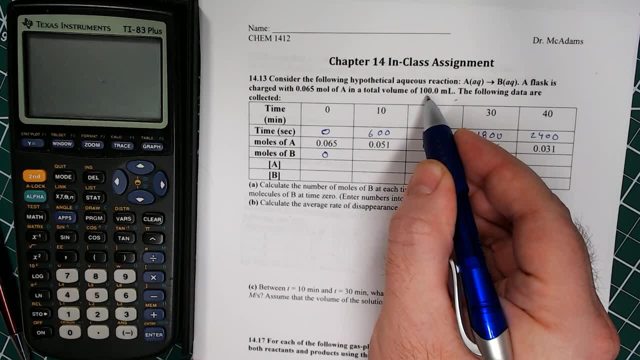 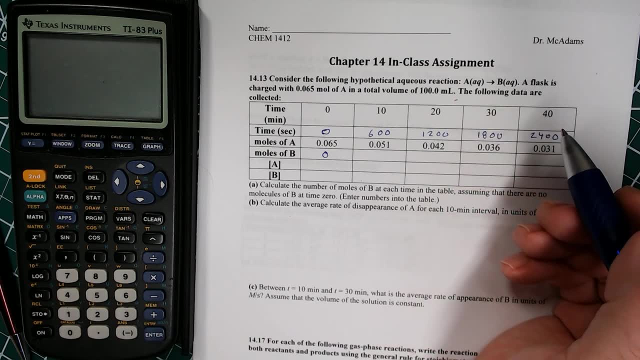 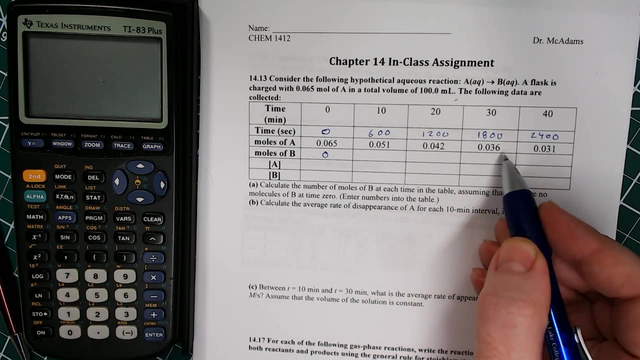 and a total volume of 100 milliliters, That's 0.1 liters for our calculation purposes. And then here these data are collected, So at 0.065, 0.051, 0.042, 0.036,. 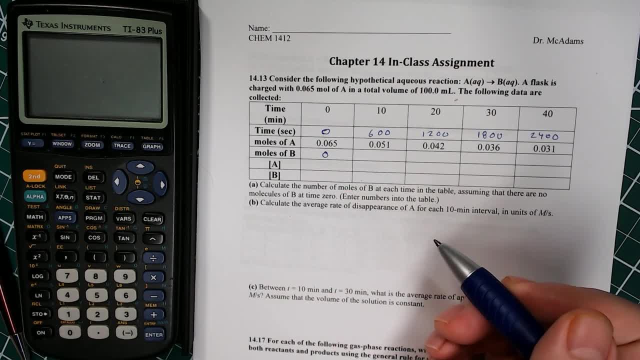 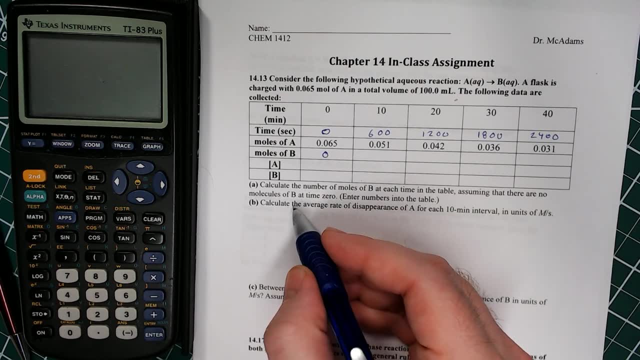 0.031 moles of A Calculate the number of moles of B at each time in the table, assuming that there are no molecules of B at time 0. So I've gone ahead and I put 0 in here for the moles of B at time 0. 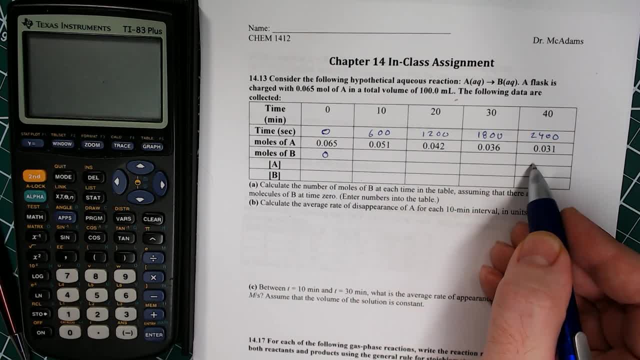 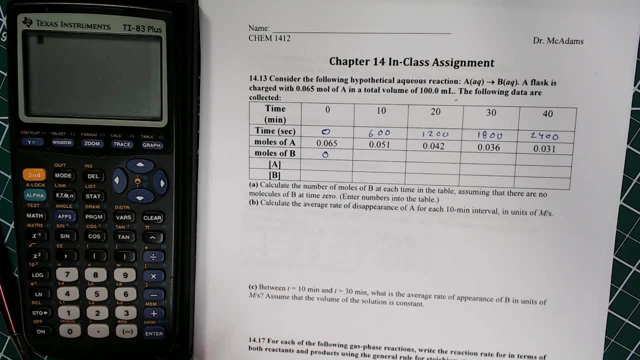 And to get these numbers, we simply need to take the difference between where we started and where we ended on. where we started and where we ended on the moles of A, Because to the extent that any A was used up, it was converted into B. 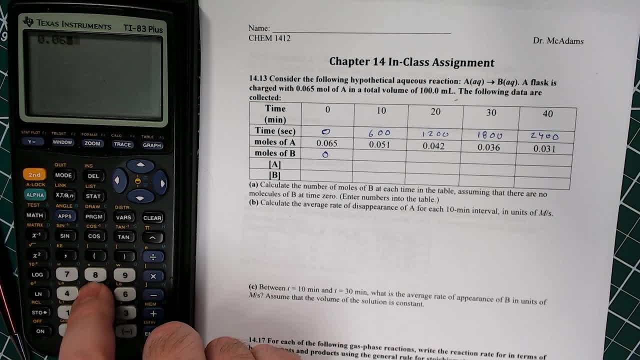 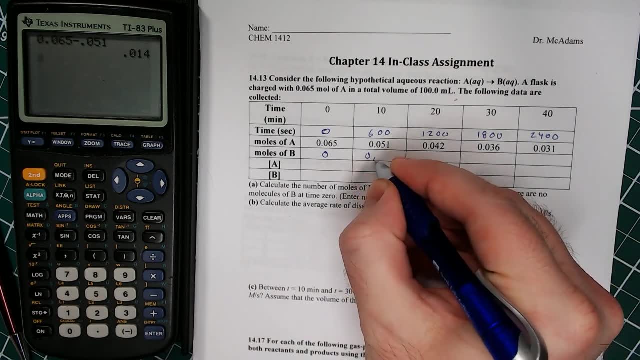 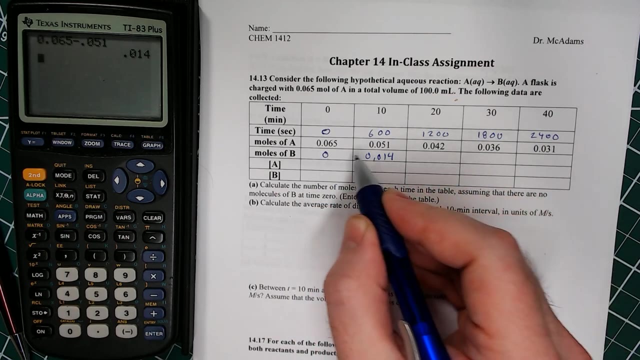 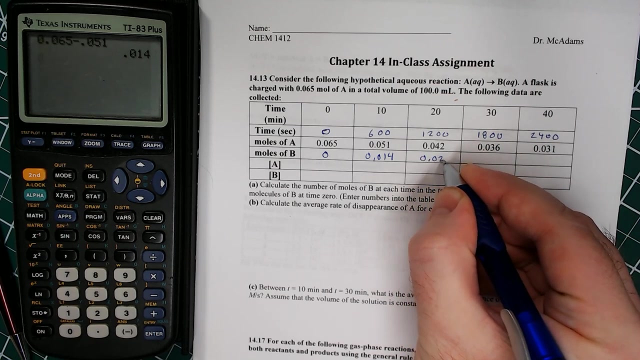 So if we do 0.065 minus 0.051, we're going to get 0.014.. And so you can see here 0.065, you can probably do these in your head. 0.065 minus 0.042 is going to give us 0.023. 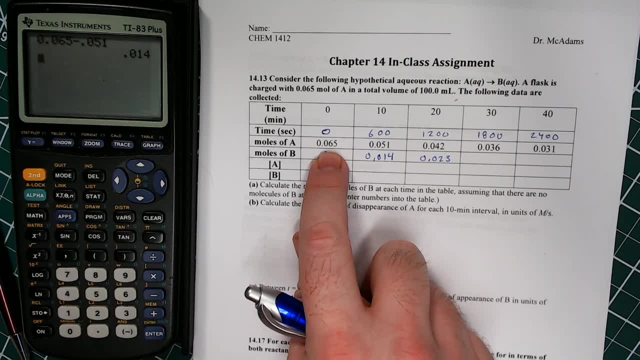 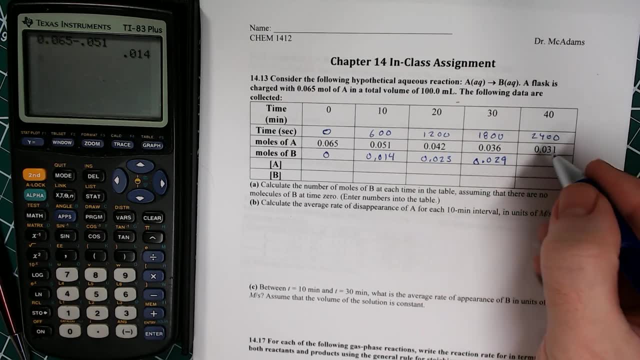 And then 0.065 minus 0.039 is going to give us 0.029.. And then, finally, 0.065 minus 0.031 gives us 0.034.. So we've got the number of moles of B. 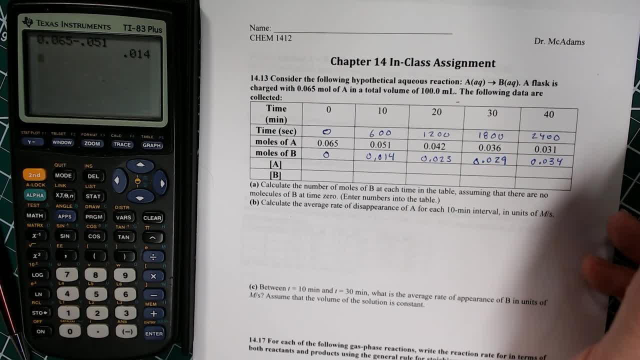 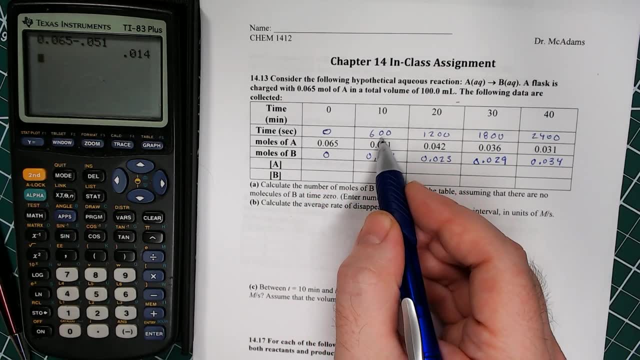 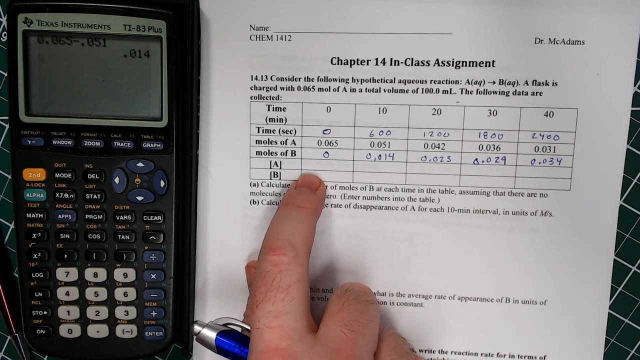 at each of those times. Now you'll also notice that I've calculated the time in seconds. I just took the time in minutes and multiplied by 60 to get each of these numbers. Since that was an easy calculation to do, I went ahead and did that. 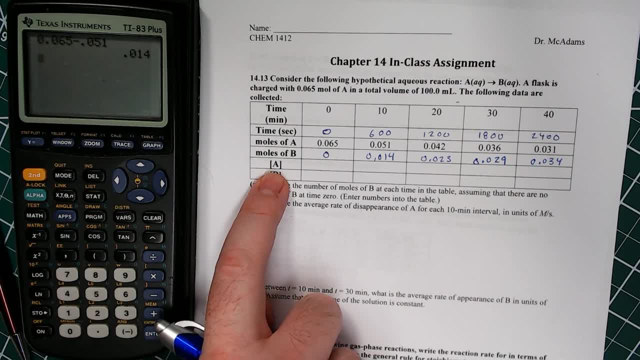 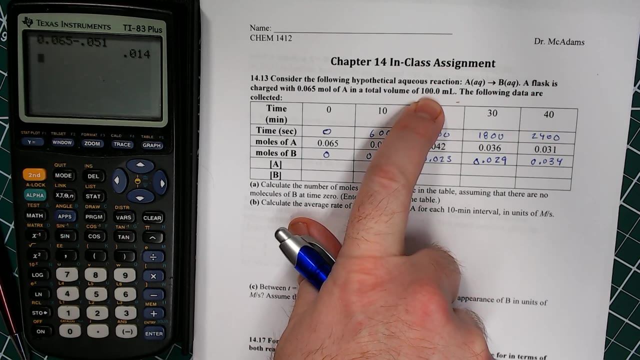 To get the concentrations, and we're going to need these concentrations before we can do Part B. to get those concentrations, we just need to divide by the number of moles of B. We need to divide by the number of liters. In other words, we need to divide by 0.1000 liters. 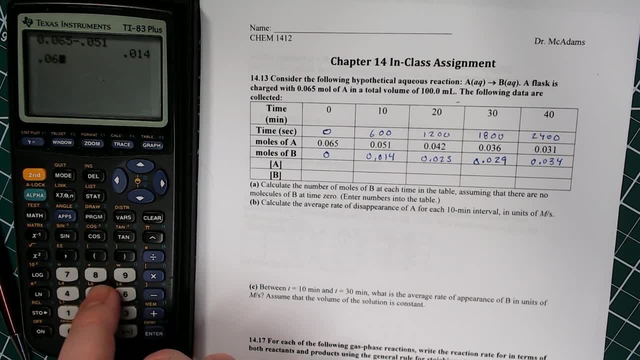 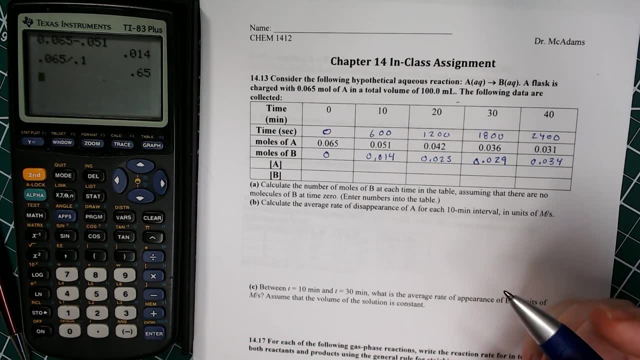 So I'm going to take 0.065 and divide by 0.1.. Now, once I do this one, you're going to see that this is a really easy calculation, that we don't need to really put these all in the calculator. 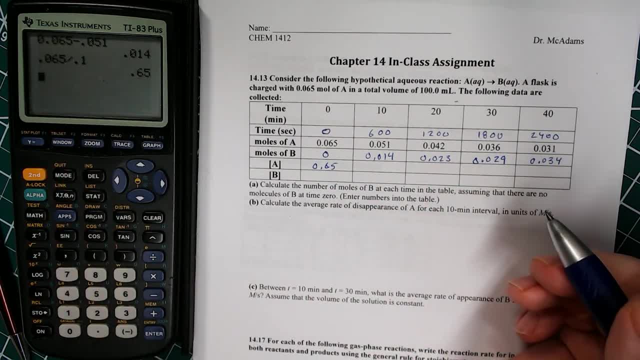 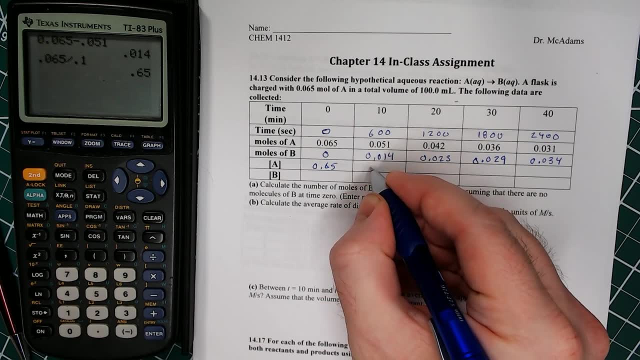 We can just write them down: When you divide by 0.1, you're multiplying by 10.. So 0.065 becomes 0.65.. 0.051 becomes 0.51.. 0.42 molar. 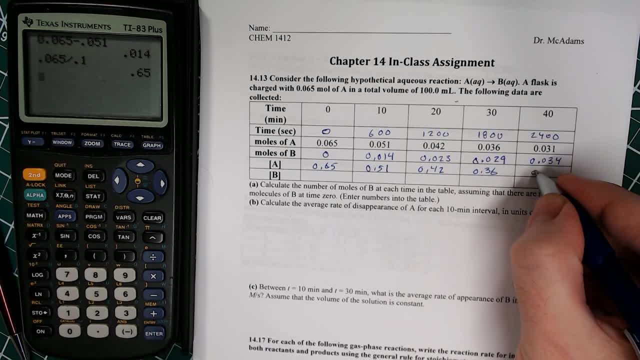 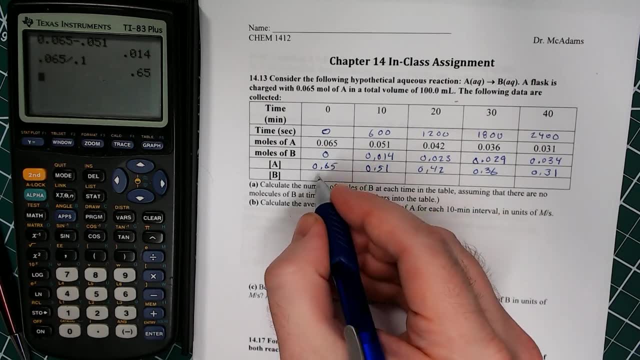 0.36 molar And 0.31 molar For the concentration of B. we'll do the same thing. So 0 divided by 0.1, of course, is 0.. 0.14.. 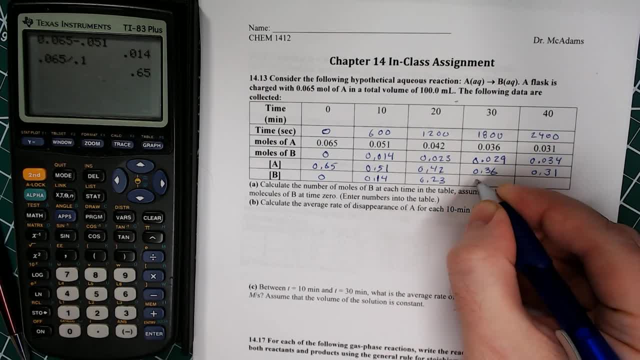 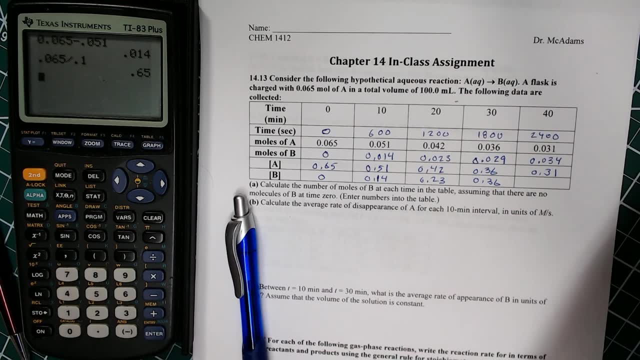 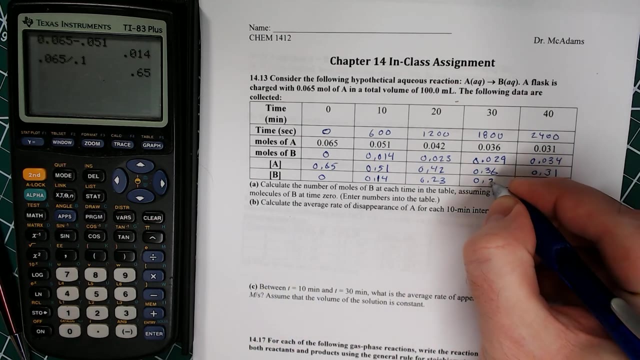 0.23.. 0.36.. 0.29.. I wrote down the wrong number there, Easy mistake, So 0.29. And finally 0.34.. So those are the concentrations of B at those time intervals. 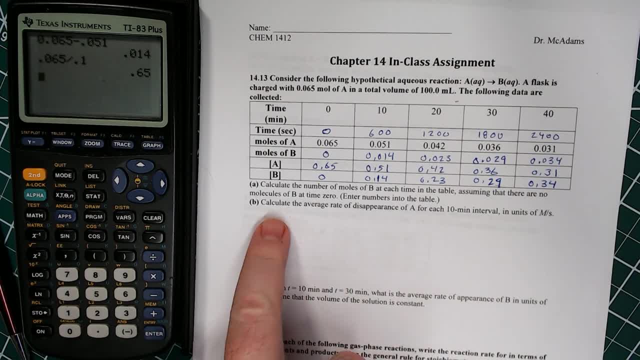 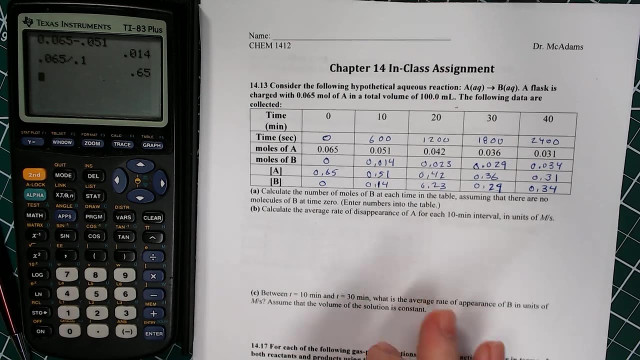 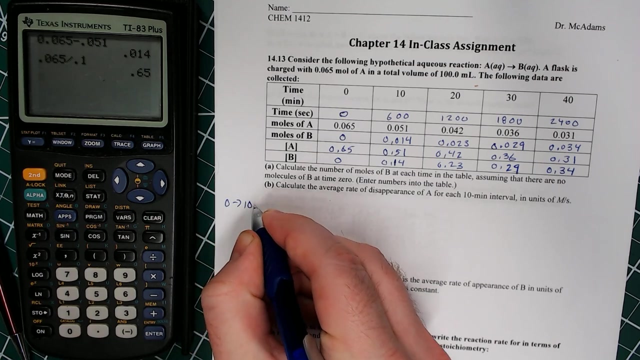 So next, we want to calculate the average rate of disappearance of A for each 10-minute interval, And so, to do this, we're going to look at each of these intervals, and we'll start from 0 to 10 minutes. 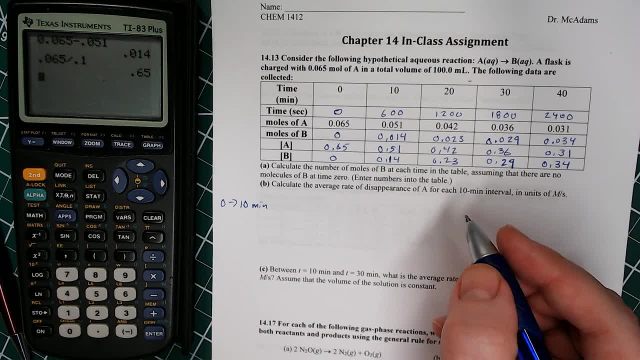 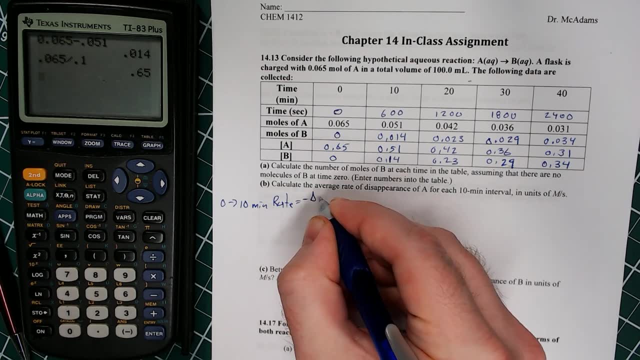 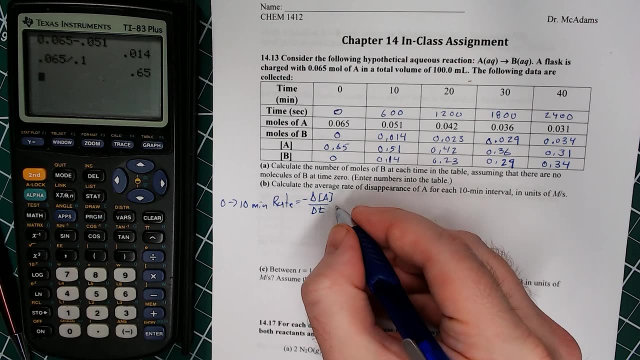 So in that time slot from 0 to 10 minutes our rate is equal to negative. the change in the concentration of A over the change in time, And we want that time to be in seconds, All right, So negative And we'll do the concentration at 10. 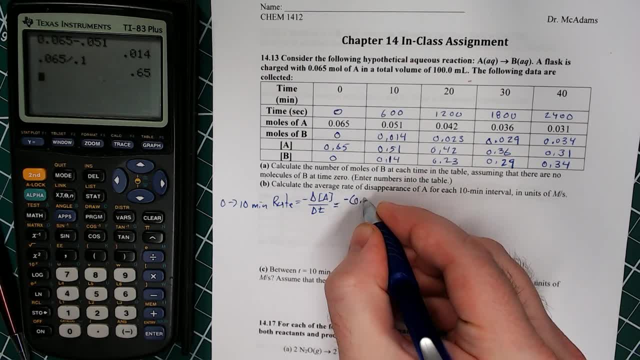 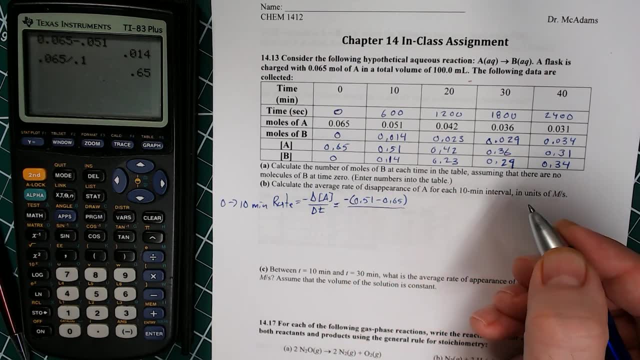 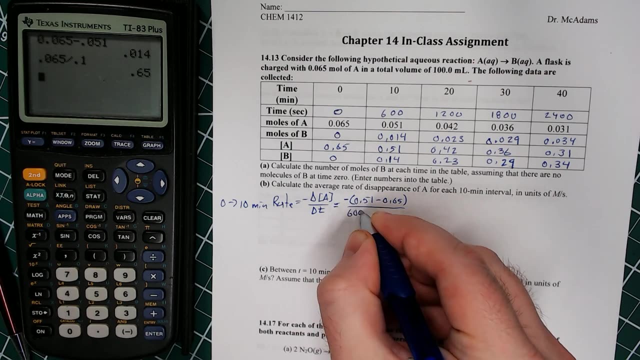 minus the concentration at 0.. 0.51 minus 0.65.. And then we will divide that by 600 seconds minus 0 seconds, And that gives us a value All right. So we'll go ahead and put that number in here. 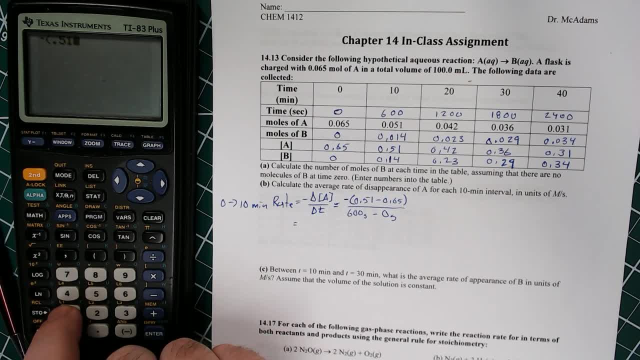 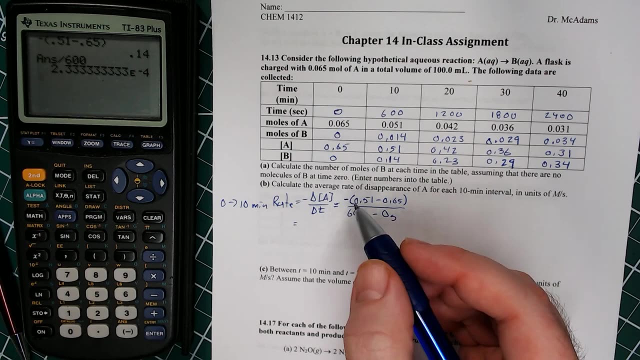 So negative parentheses: 0.51 minus 0.65, close parentheses, And then we will divide by 600 minus 0, which is just 600.. And then that gives us 2.3333 times 10 to the negative 4.. 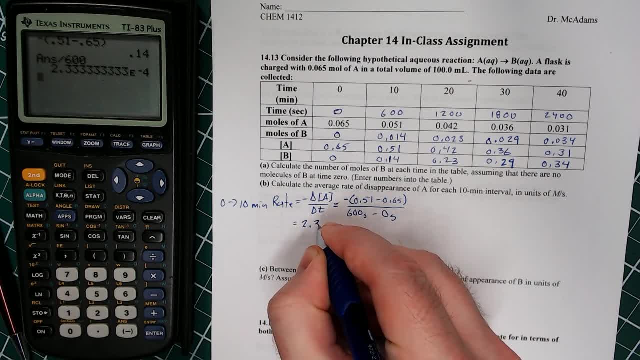 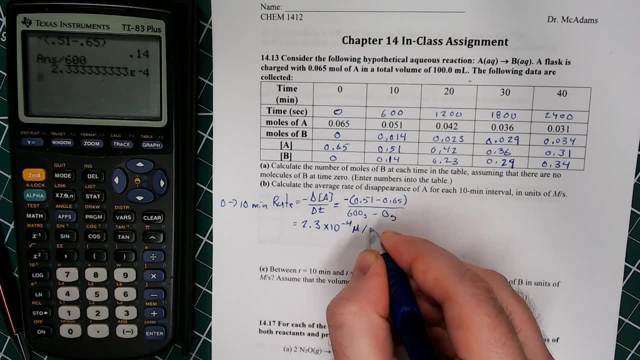 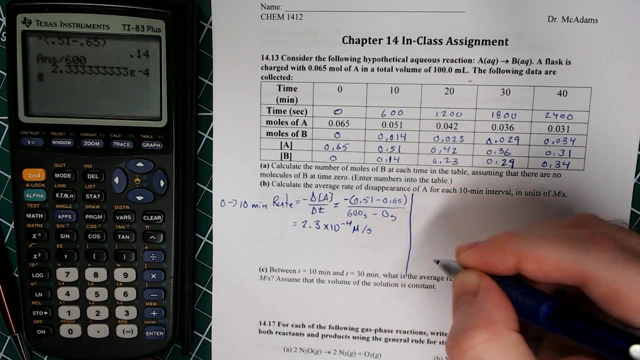 We're just going to do two sick figs here and call it 2.3 times 10 to the negative 4 molar per second. All right, So that is our rate for the first 10-minute interval. So now let's do 10 to 20 minutes. 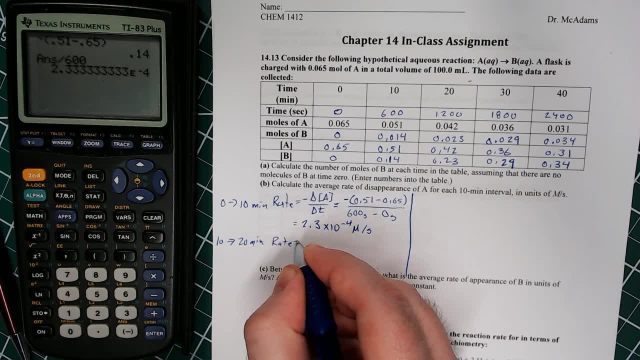 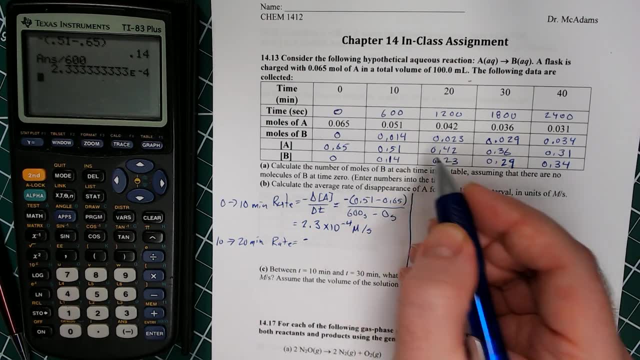 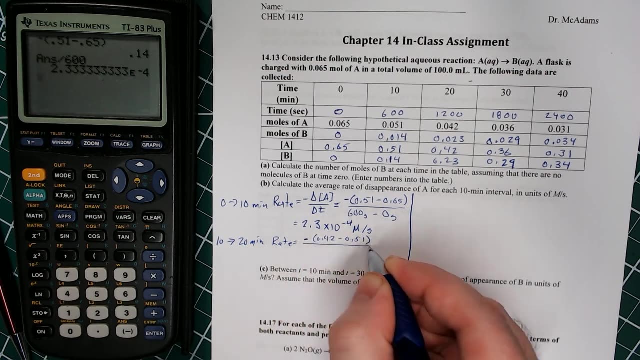 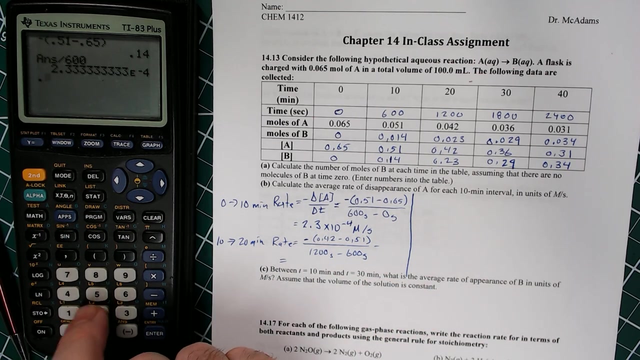 All right, So our rate. it's the same formula here, So our rate is negative. let's see 0.42 minus 0.51.. Over 1200 seconds minus 600 seconds, All right, So point. 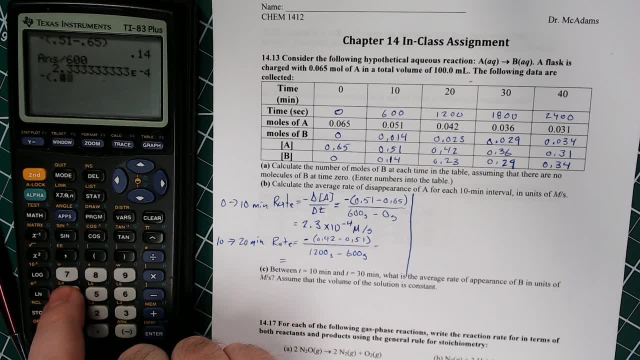 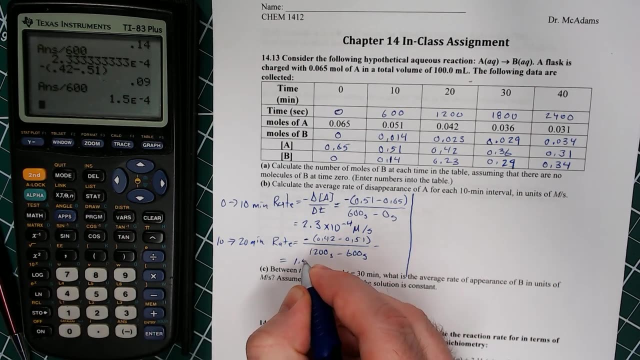 so negative parentheses: 0.42 minus 0.51, close parentheses, And then 1200 minus 600 is 600. So we'll do divide by 600. And that's going to give us 1.5. 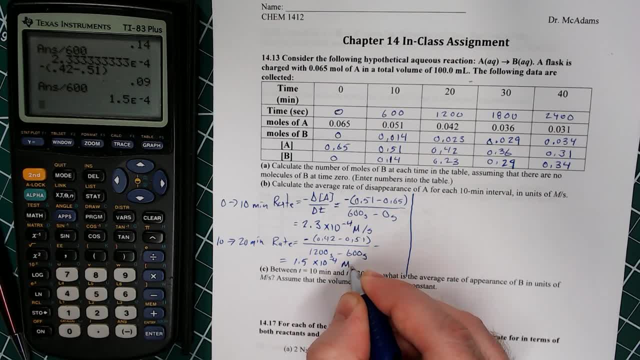 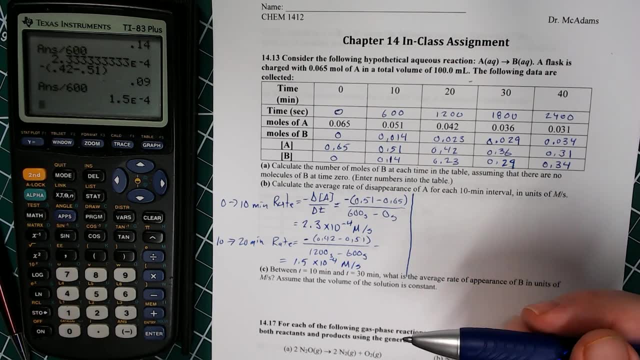 times 10 to the negative 4 molar per second. Now, not surprising. you'll see that the rate of reaction went down. That is exactly what we would expect to happen. So now let's do the interval from 20 minutes. 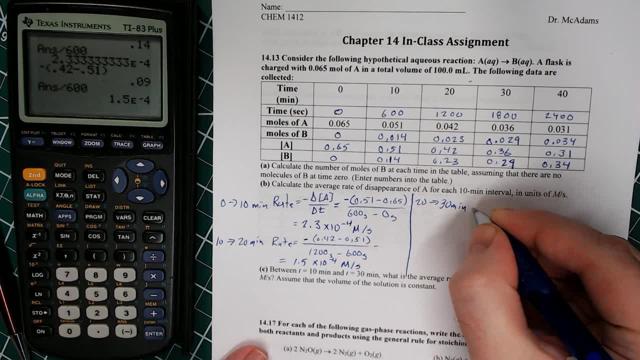 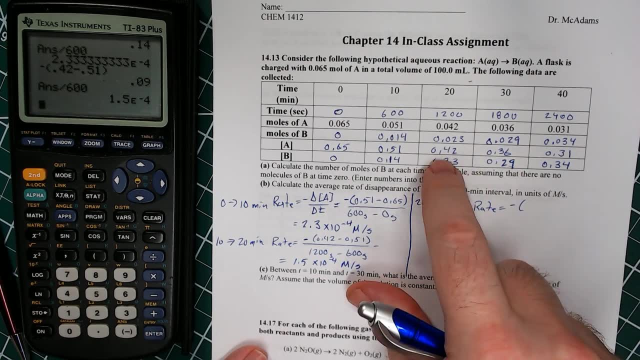 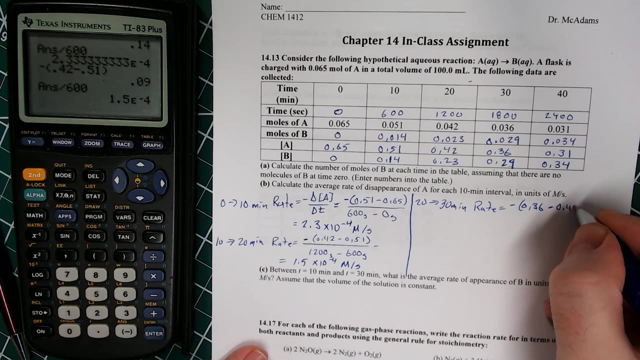 to 30 minutes. All right. So our rate so negative. we'll do 0.36 minus 0.42.. So 0.36 minus 0.42.. And then we'll do 1800 minus 1200.. 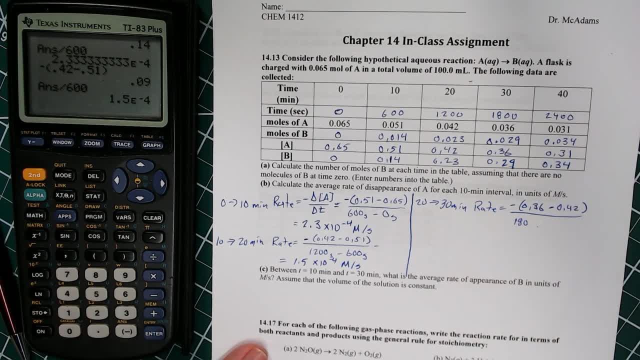 Now 1800,. I left a 0 off there, So I'll fix that real quick. So minus 1200 seconds, All right. So negative 0.36 minus 0.42, close parentheses, And then we're going to divide that by 600 seconds. 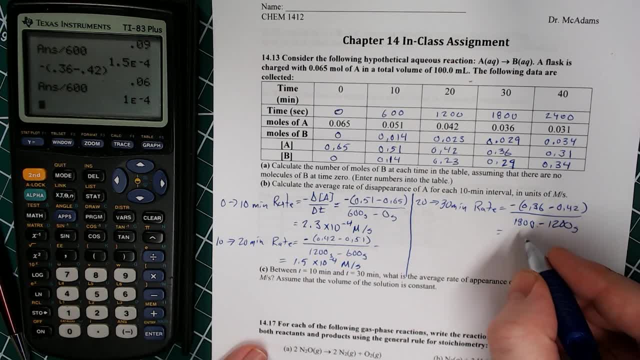 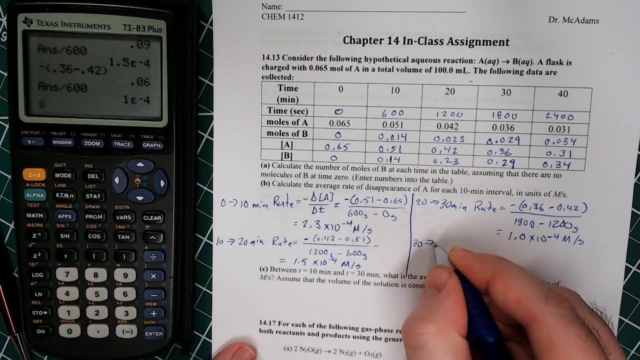 Again, 1800 minus 1200 is 600 seconds And you'll see the number we get. there is 1.0 times 10 to the negative 4 molar per second. All right. Finally, from 30 to 40 minutes. 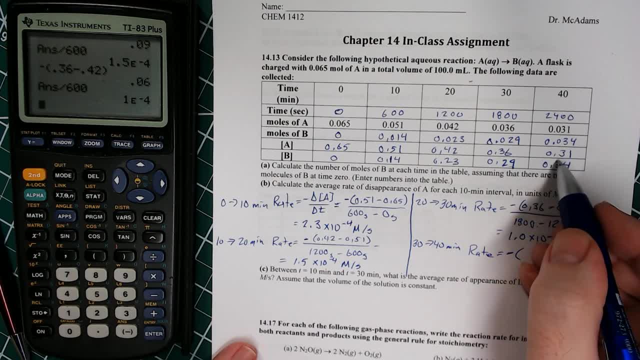 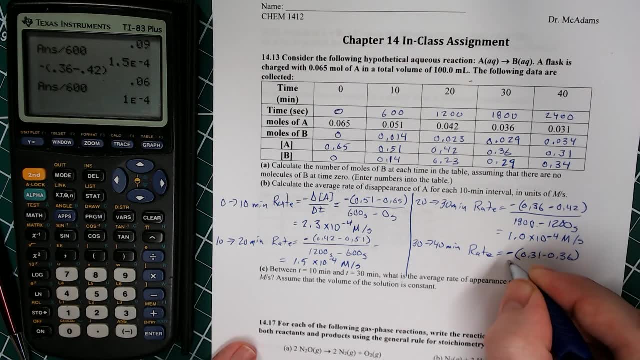 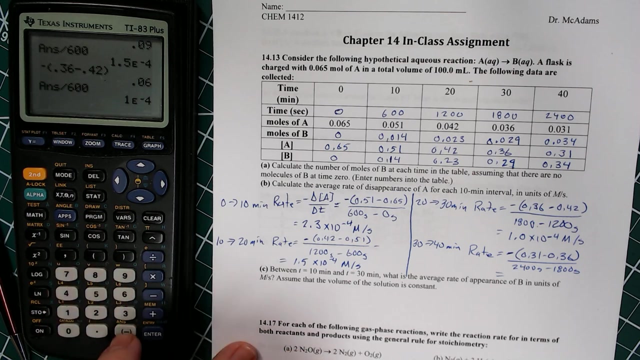 And here the rate 0.31, 0.36.. So 0.31 minus 0.36.. And then 2400 seconds minus 1800 seconds, All right, And so negative 0.31,. 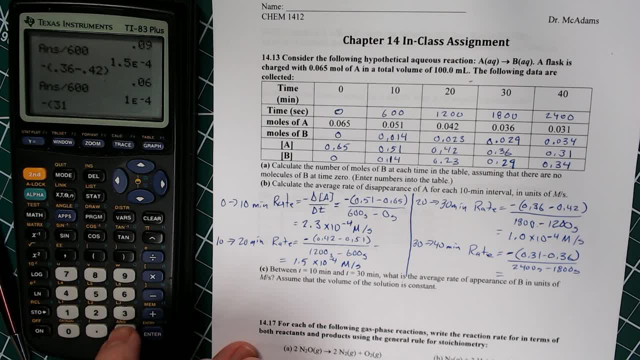 oh, got to put those parentheses in. So 0.31 minus 0.36.. And then we're going to divide by again: 24 minus 2400 minus 1800 is 600.. So divide by 600.. 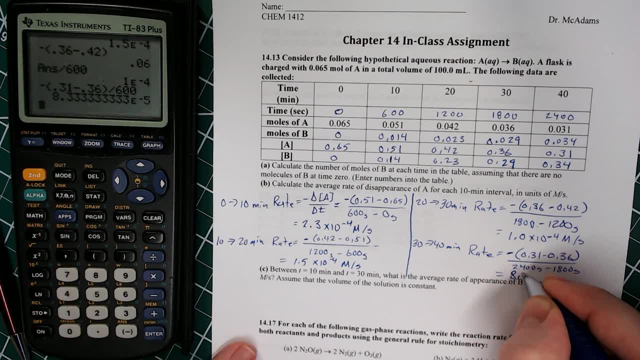 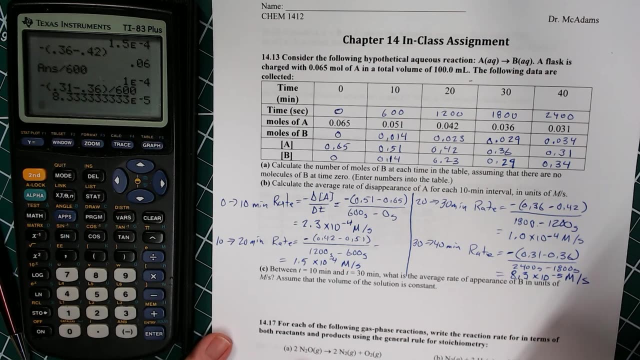 And the number that we get there is 8.3 times 10 to the negative: 4 molar per second. Times 10 to the negative: 5 molar per second. All right, So we definitely see that the rate of this reaction decreases as time goes on. 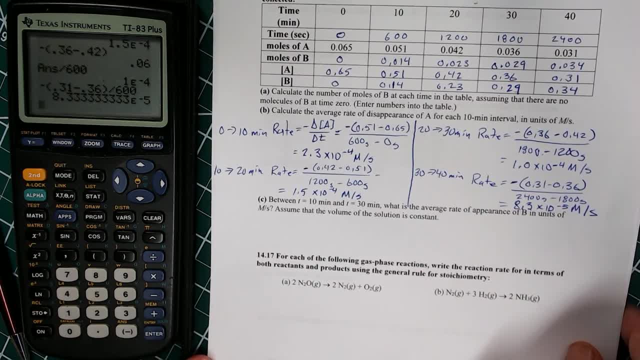 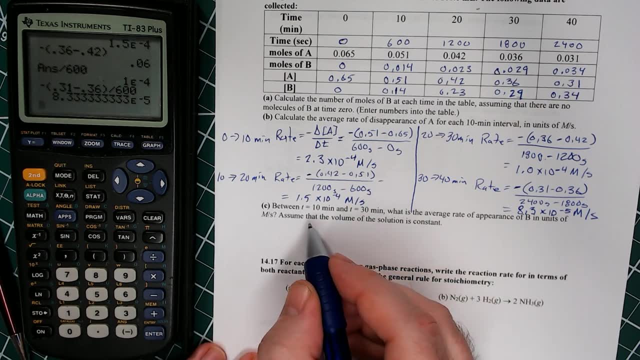 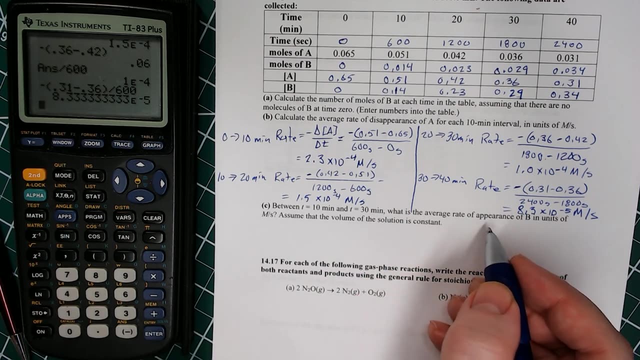 We have one more part of this problem that we want to do And with this one more part of the problem we want to, with this one more part of the problem, we want to. between 10 and 30 minutes, what is the average rate of appearance of B? 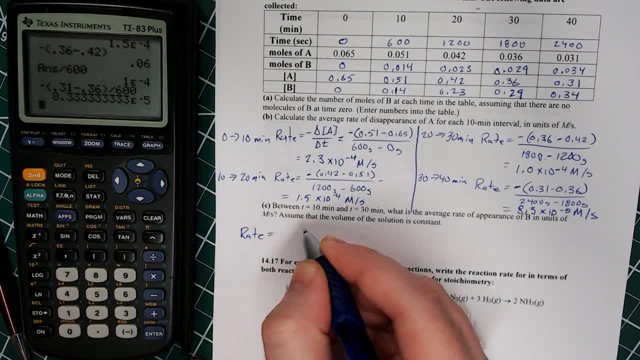 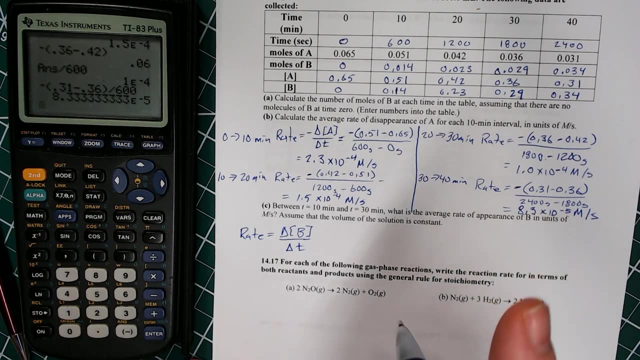 Well, here the rate is going to look a little bit different. Instead of being negative, it's going to be the positive: the change in the concentration of B over change in time. The reason that it is positive is because it is a product. 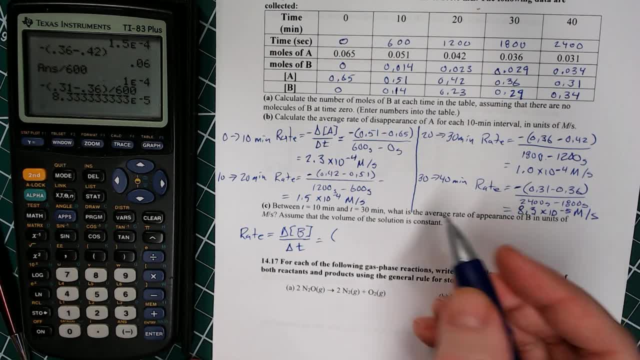 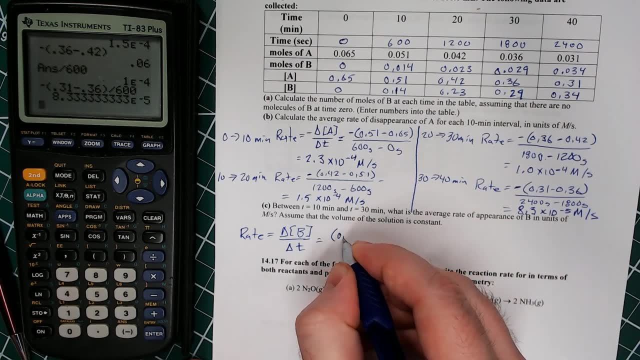 So at, let's see, from 10 to 30 minutes. So our concentration of B at 30 minutes was 0.29 molar, Minus at 10 minutes it's 0.14 molar. 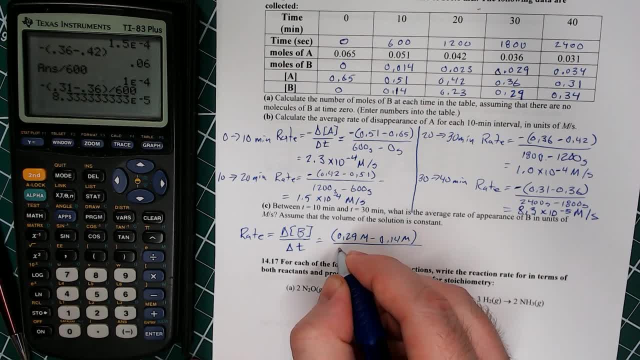 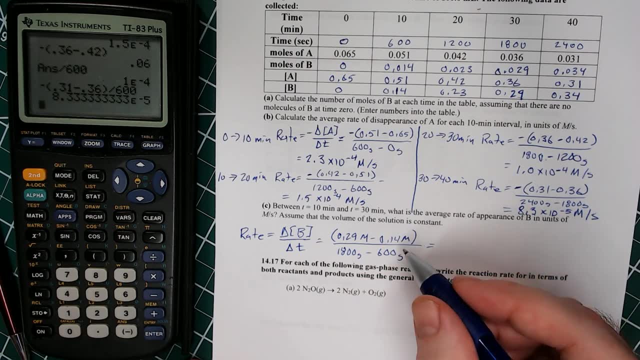 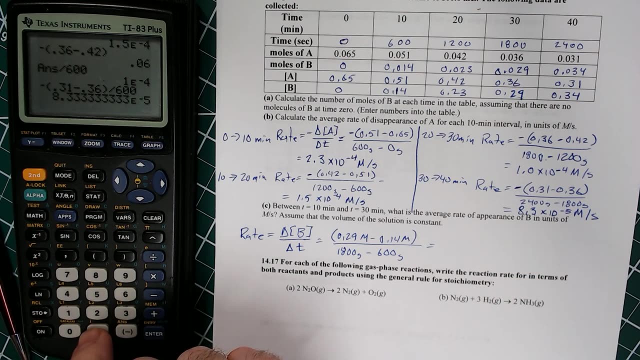 And then our time was 1800 minus 600.. So 1800 seconds minus 600 seconds, And I put the units in here so that you can clearly see that the answer is going to be in molar per second. So 0.29 minus 0.14. 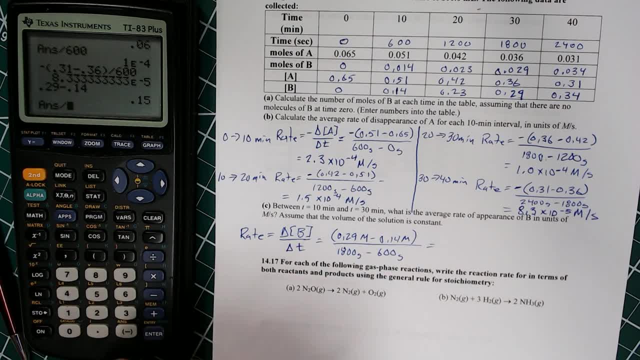 So that gives us 0.15.. And then we're going to divide that number by 1800 minus 600, which of course is 1200.. We could have just punched that in, But you'll see the number that we get there is 1.25.. 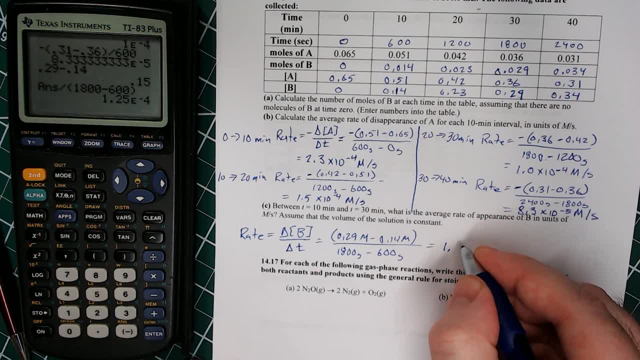 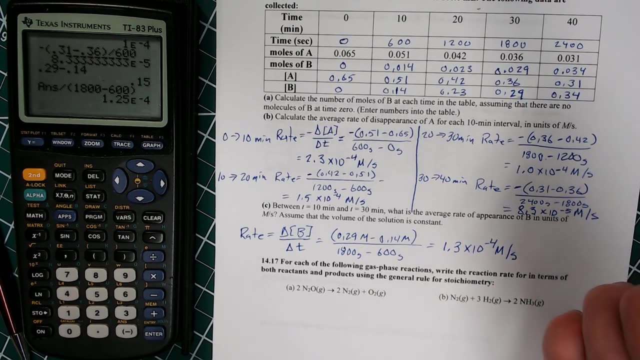 I'm going to go ahead and round that to two sig figs And call it 1.3 times 10, to the negative 4 molar per second. All right, So now I have shown you how you can calculate the rate. 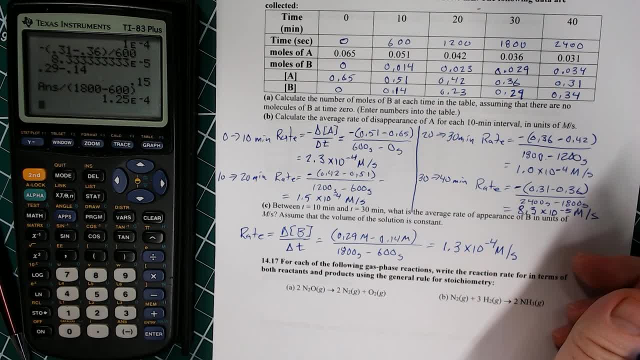 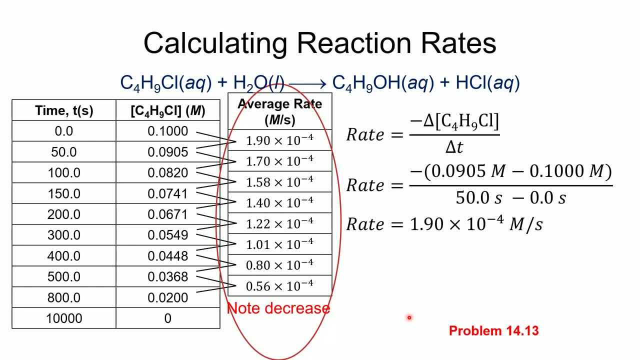 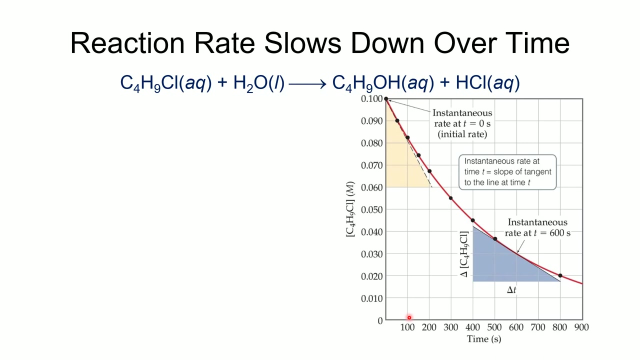 using just raw data like this. Okay, So I did. I did mention that the rate decreases as time goes on, And so we want to look at what does that mean, Like what does that mean and how can we represent that. 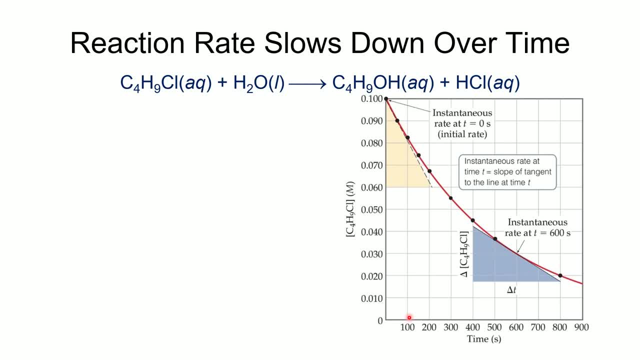 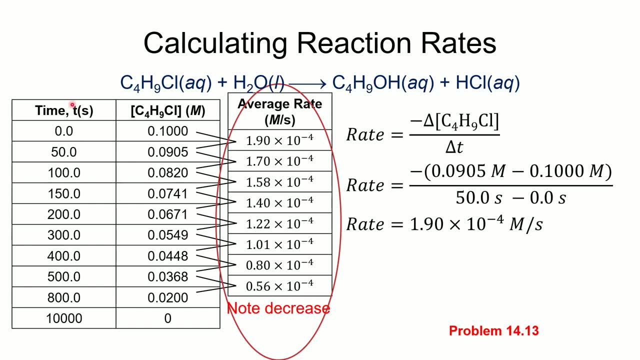 Well, we can represent that by looking at a graph. We can plot the data. I'm going to go back to that data that we just had. We can plot this data. So on the x-axis we put the time And on the y-axis we put the concentration. 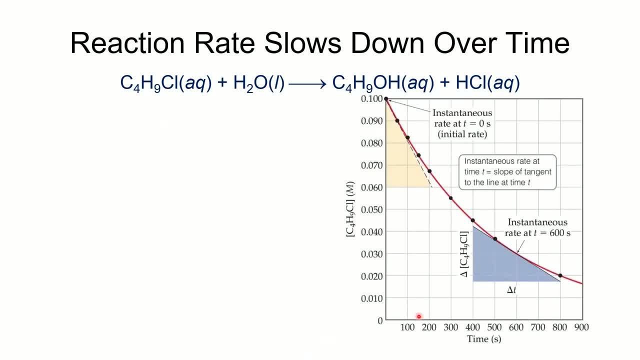 And when we do that, we will get this. So here's our x-axis with time, There's our y-axis with the concentration And our y-axis with the concentration, And that's our concentration versus time. Well, there's more information here. 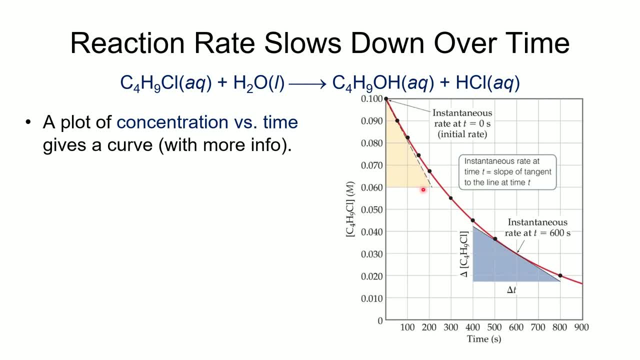 First of all, it's a visual representation of what's going on And it gives us more information. It turns out that we have calculated the slope between two points by doing these rate calculations. We calculated the slope between any two points, And that tells us what the rate is between any of those two points. 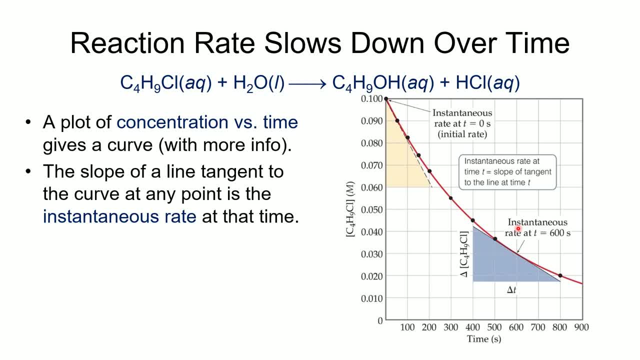 Now, what's really cool about this is we can even get rate information at points where we didn't. We didn't make a measurement, As long as we have a very accurate curve here and if we're capable of drawing a tangent line to any point. 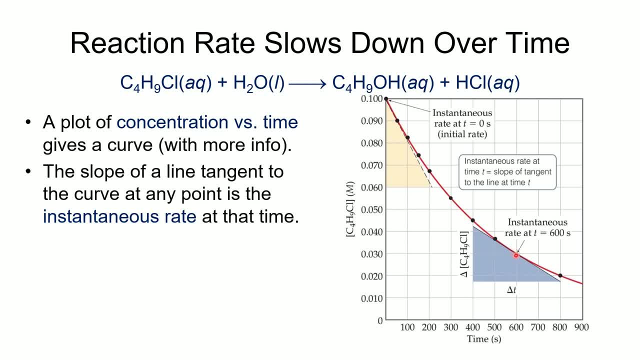 then we can get the rate of the reaction at that point, even though we don't have any data, simply by getting the slope of that line. Now, that's a little bit easier said than done when we're doing this on paper, But if you're doing it on a computer it's not too hard. 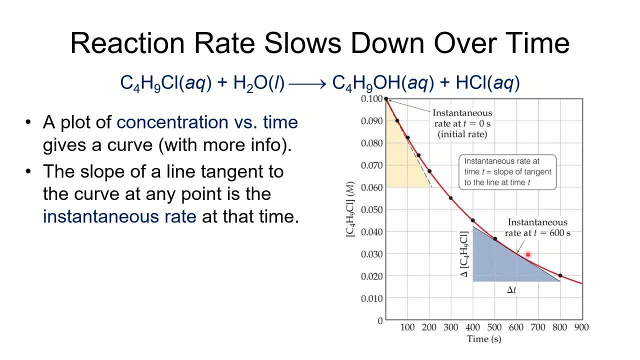 So we can get the instantaneous rate. Well, when we look at this, we can clearly see that the rate of reaction changes as time goes on, So that means that we need to decide what is the best point along that curve to get the rate. 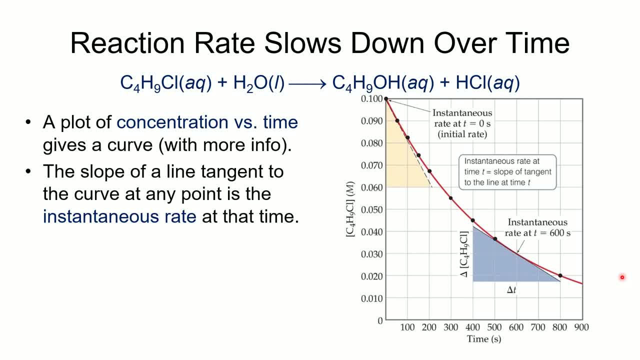 What's the most representative rate for this reaction? And it turns out, by getting the instantaneous rate, the tangent line, at zero, the instantaneous rate at zero, that that is going to give us the initial rate and that is the value that we're usually the most interested in. 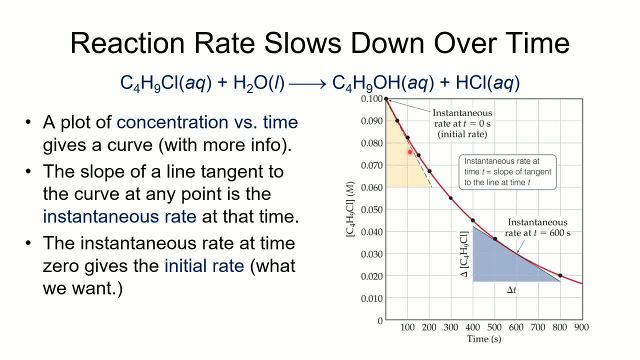 is that initial rate of reaction? All right. So later, when we're looking at rate data, we're going to be looking at initial rates. So we are going to be looking at initial rates, All right. So I want to do one more thing here before we stop this video. 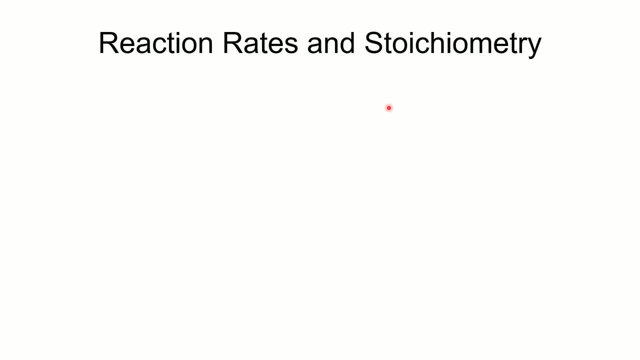 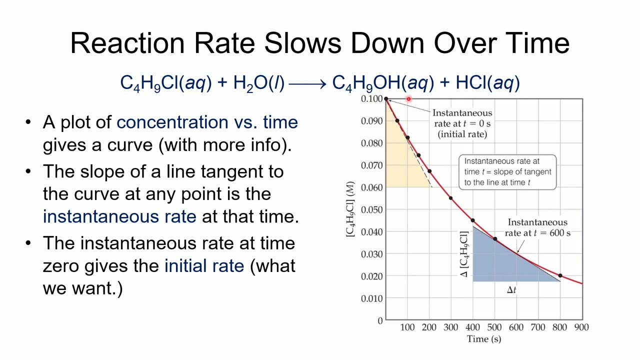 and that is to look at reaction rates when we have stoichiometry that are not one-to-one. Just to point this out, you'll notice that in this reaction all of the coefficients in that reaction are one. So that means writing the rate. for these writing, calculating the rate is really really easy. 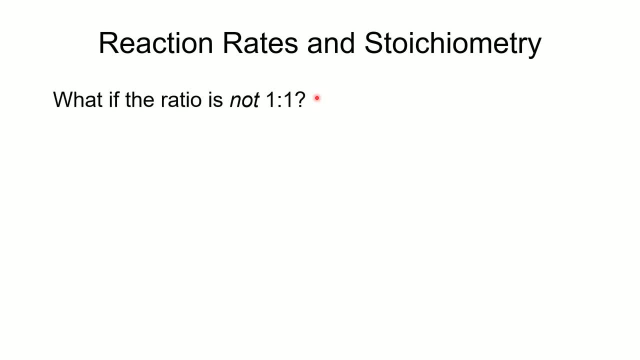 However, if the ratio is not one-to-one, then we can get the rate of the reaction by slightly modifying our equation to look like this: So again, negative indicates that we have a reactant positive for the product, But you'll notice that we took the coefficient and took its reciprocal. 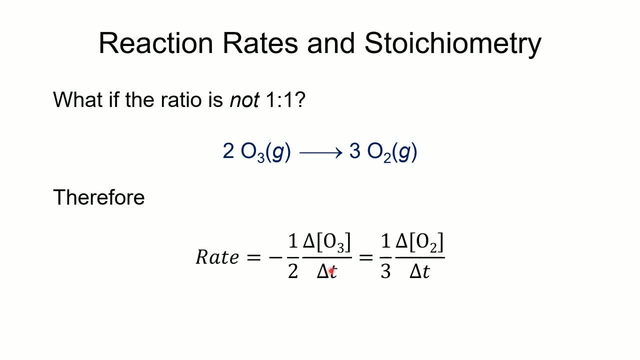 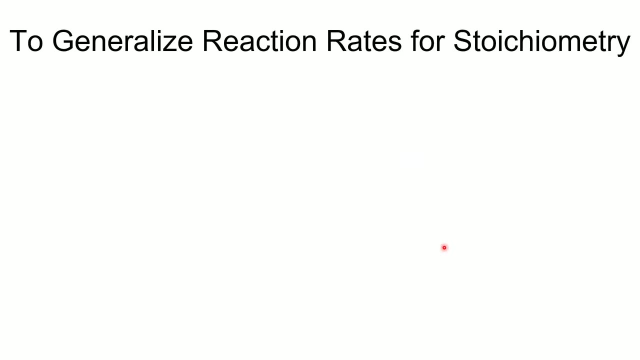 and put it in front of our delta concentration over delta time. And so one over two, one-third here for this product, All right, And we can generalize this. We can generalize this using this particular one, All right. So here our coefficients are the lowercase letters. 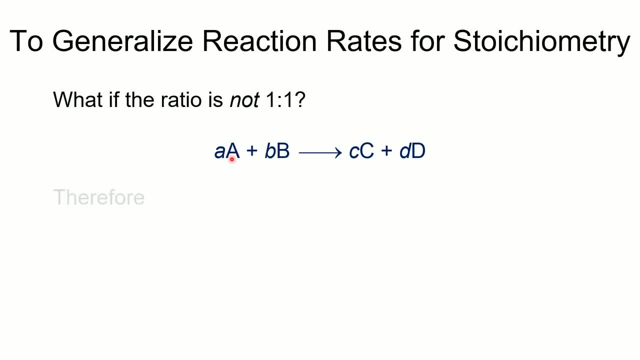 and the chemicals are the uppercase letters, And so we can write the rate law or not the rate law, but we can write the rate of a reaction, again negative for the reactants, positive for the products, and it's just one over the coefficient to give us a normalized value for those rates. 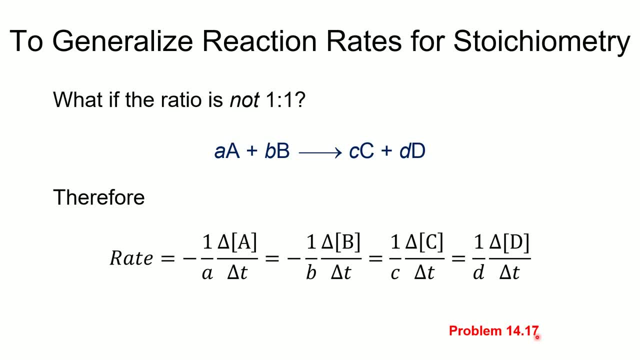 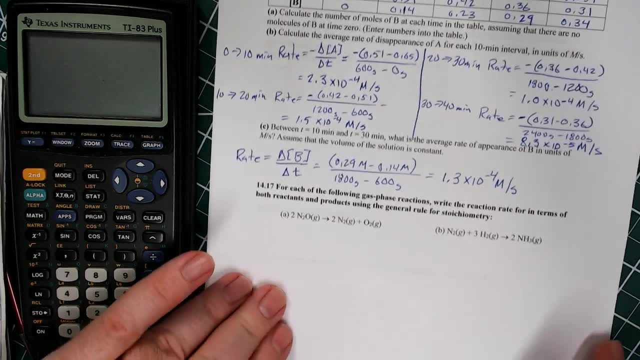 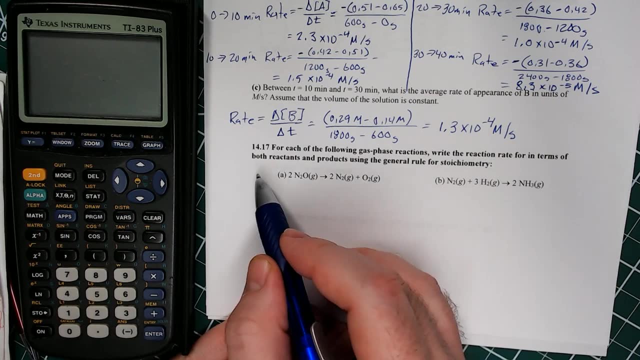 So we're going to look at number 17 on the in-class assignment, And this is a relatively easy problem. All right, So for each of the following gas phase reactions, write the reaction rate in terms of both reactants and products. 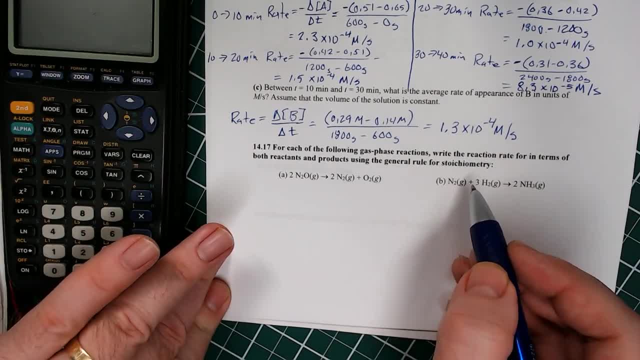 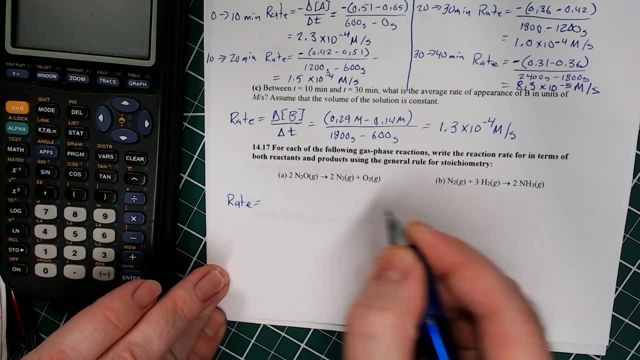 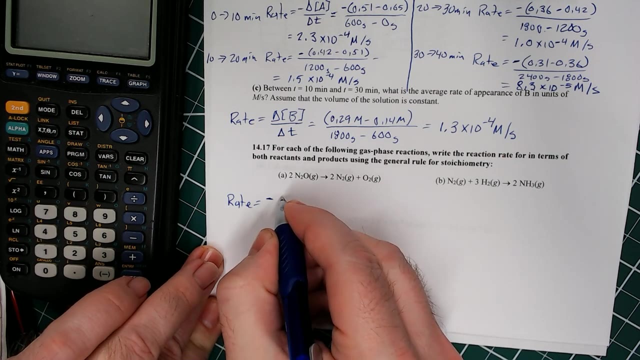 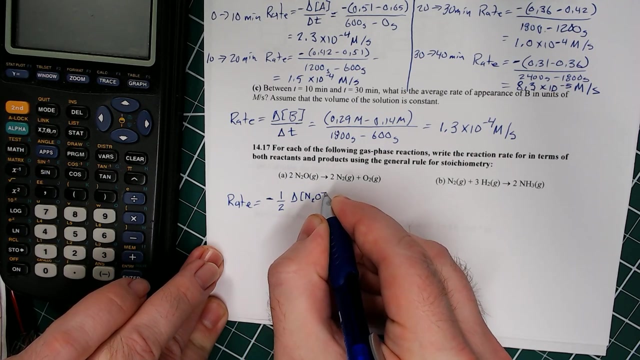 using the general rule for stoichiometry. So our general rule for stoichiometry again, rate is here. we've got a reactant, so we're going to put a negative value out front. Since the coefficient is two, we'll put one over two. delta concentration of N2O over delta T. 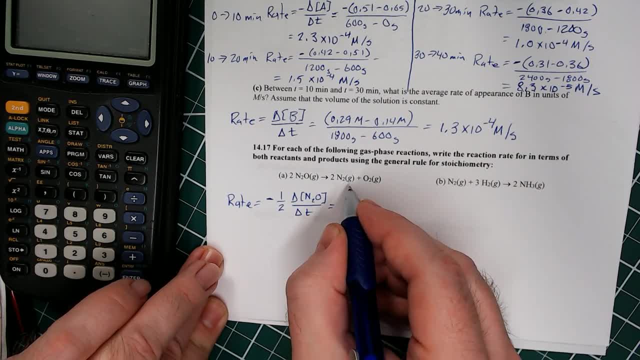 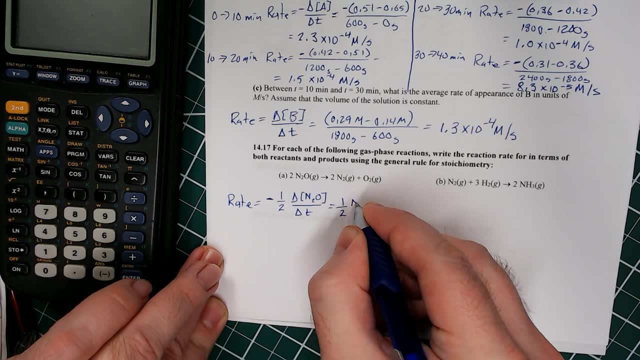 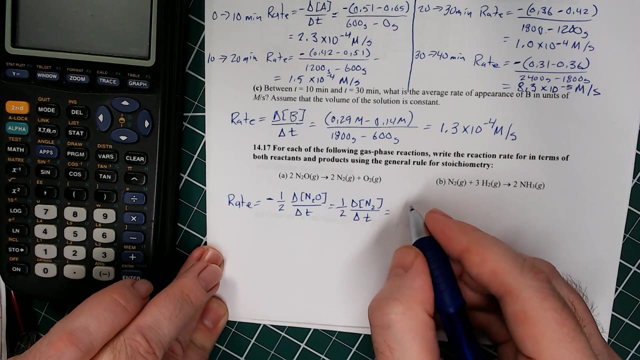 Here for nitrogen again. since this one's a product, we're going to leave it as positive. But we do have a two there, so we're going to put one half the delta concentration of N2 over delta T. And then, finally, for the oxygen. 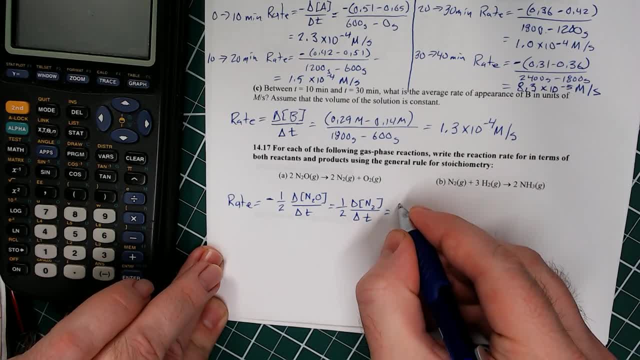 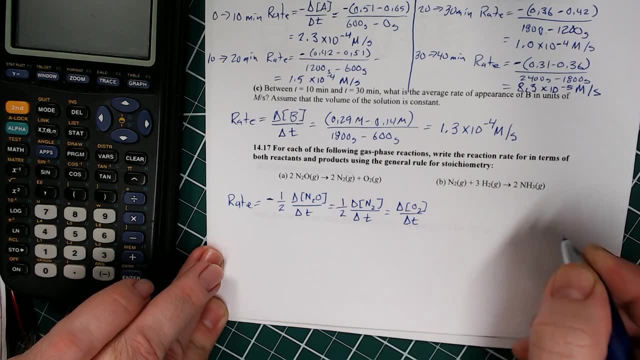 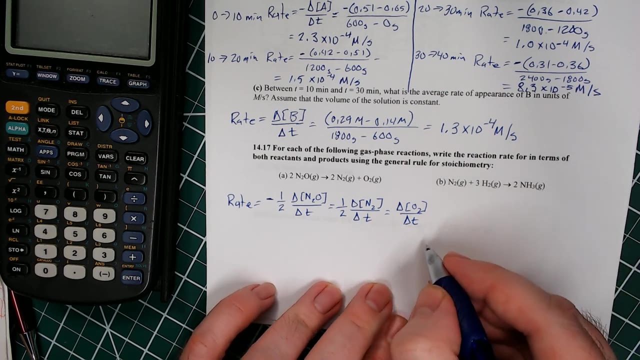 it's a product, so it's positive, and the coefficient is one. so here we just need to put delta O2 over delta T. All right, Now for this one. We've got nitrogen hydrogen and ammonia, So I'll scoot this down a little bit. 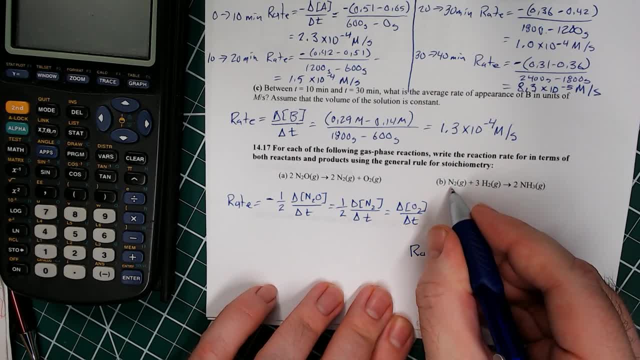 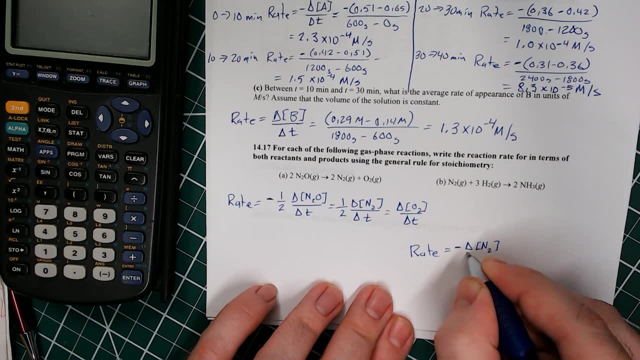 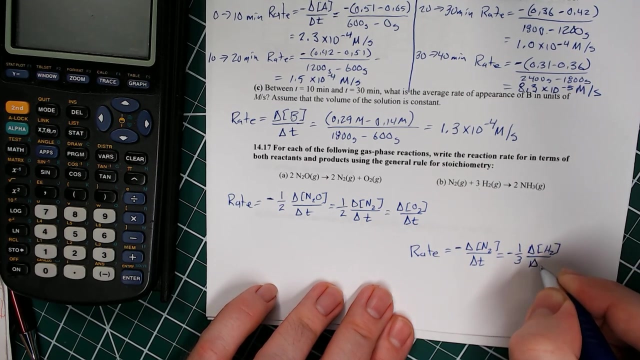 So the rate is equal to. this one's going to be negative because it's a reactant. so we'll put negative delta N2 over delta T And then this one's also reactive, but it has a coefficient, so negative one-third delta H2 over delta T. 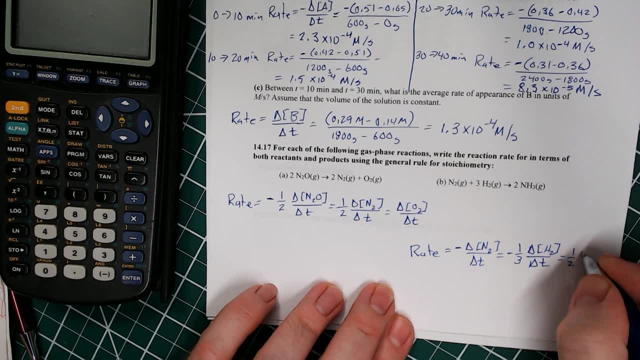 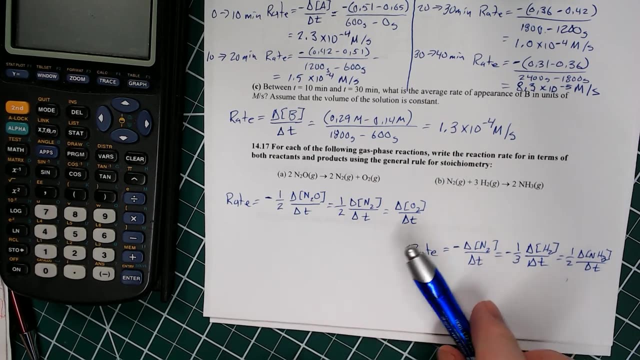 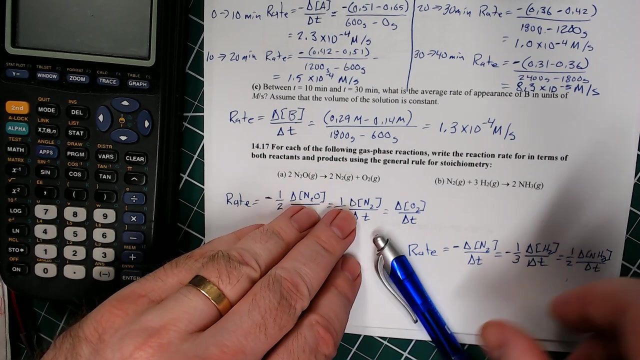 And then finally, one-half delta NH3 over delta T, And so now we've got the reaction rates for these. So I do want you to know how to do that, All right? Well, I'm going to stop this video and we'll start up the next video talking about how concentration affects the rate.